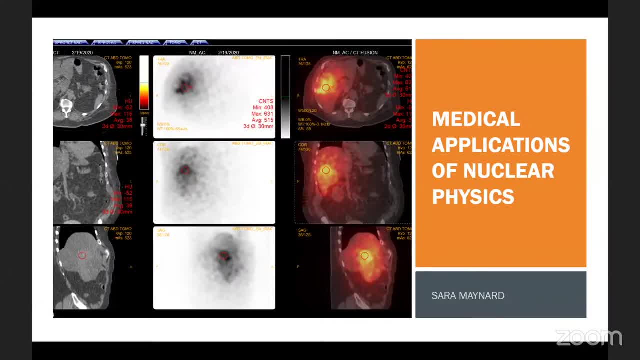 All right, I think we're live on YouTube. So, Peter- I think I mean Christian- does everything look good on your end? I'm going to check the stream on the web right now. It's looking good on my end. 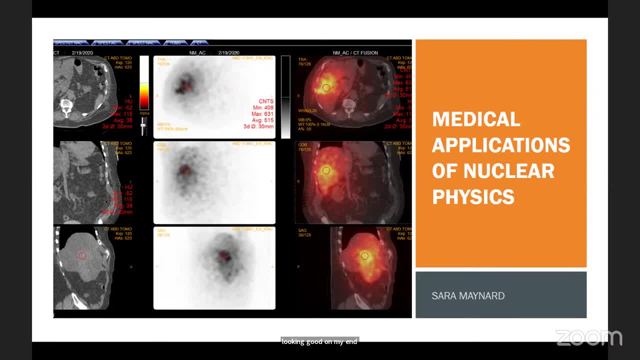 Yeah, it looks good on my end. Okay, then we can go. Yeah, I would say, Peter, you're in charge. Some people might trickle in, but you can. I think you're welcome to go ahead and get started. 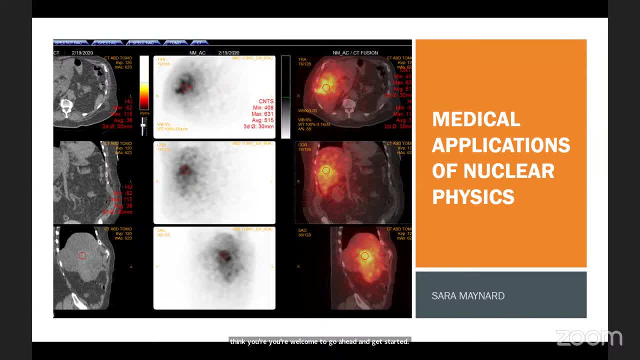 Great, thank you. So good afternoon and welcome virtually to Old Dominion University and its remote experience for young engineers and scientists. I'm Peter Mollica, I'm an assistant professor in medical diagnostics and translational science and I'm a member of the RAIS team here at ODU. 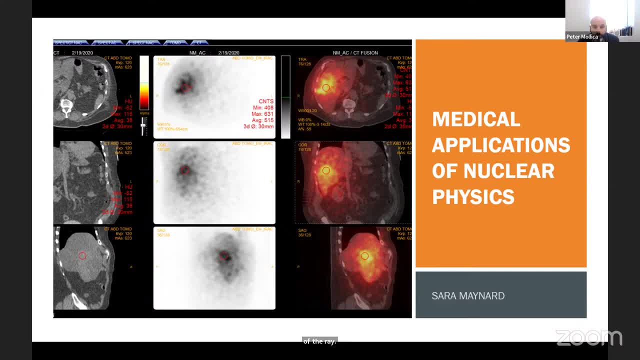 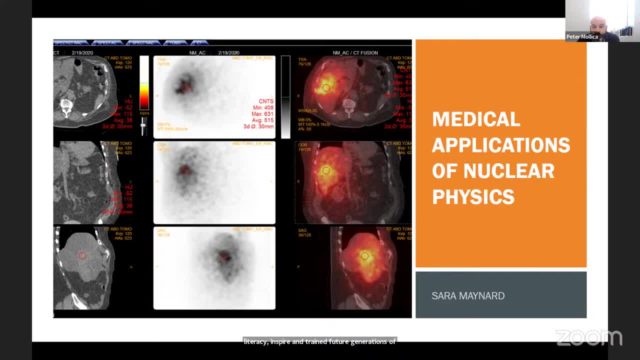 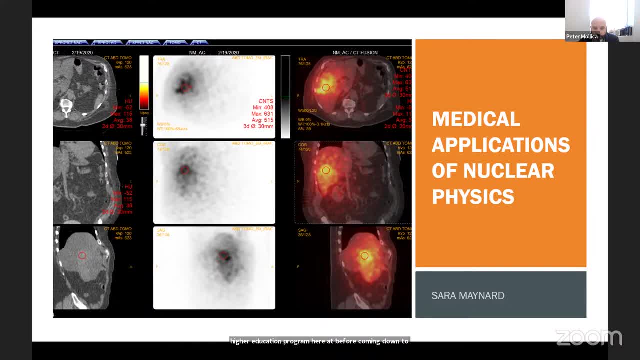 Before coming to ODU, Sarah worked in Nuclear Medicine, PET CT and Diagnostic CT at Sentara Healthcare and the Hampton University Proton Therapy Center and still remains active in the field at Sentara Healthcare. She is excited to share her experience and passion for the field with Cronkite. 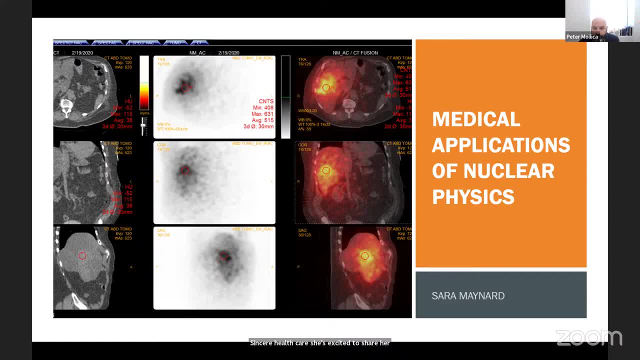 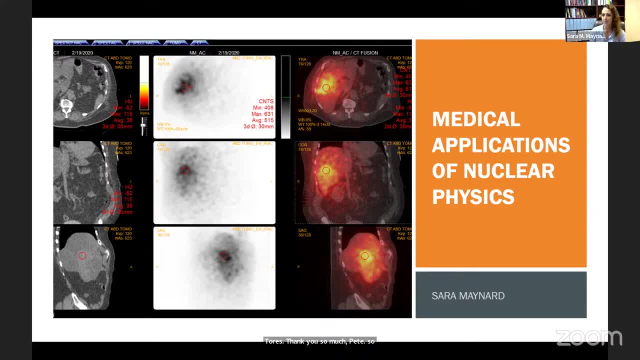 Thank you so much, Pete. So my name is Sarah Maynard. Today we will be discussing medical applications of nuclear physics. I actually brought some images from my clinical practice to share with you all today, So I'm really excited to share my passion for nuclear medicine. 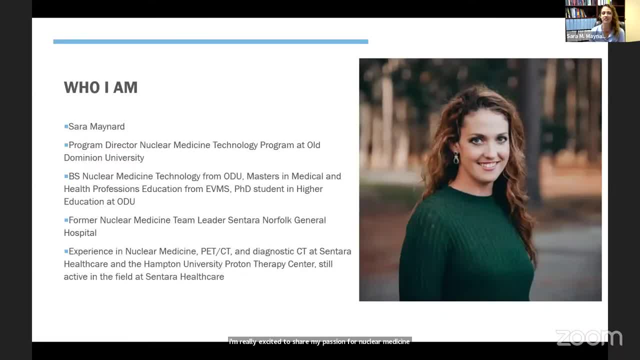 So, as Pete already introduced me, my name is Sarah Maynard. I'm the program director and a clinical assistant professor at Old Dominion University in the nuclear medicine technology program. I graduated from the ODU nuclear medicine technology program at ODU, which is really exciting to be back. I have a master's in medical and health professions. 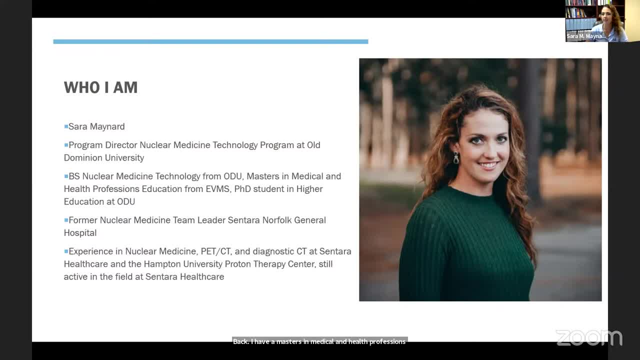 from Eastern Virginia Medical School and I'm currently a PhD student here at ODU. I've spent the majority of my career clinically in nuclear medicine, positron emission tomography and diagnostic computed tomography at Sentara Healthcare and at the Hampton University Proton. 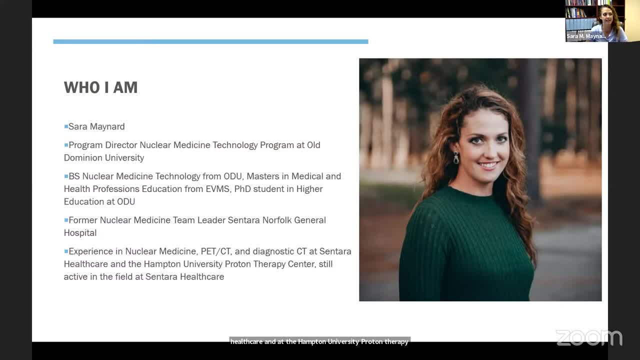 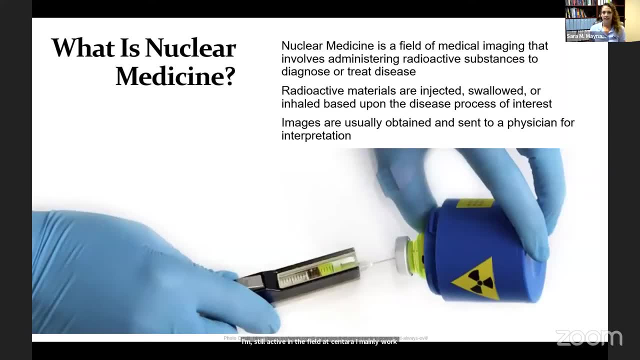 Therapy Center. I'm still active in the field at Sentara. I mainly work in nuclear medicine and in PET-CT. So many of you may be familiar with me. I'm Sarah Maynard and I'm the program director at ODU. 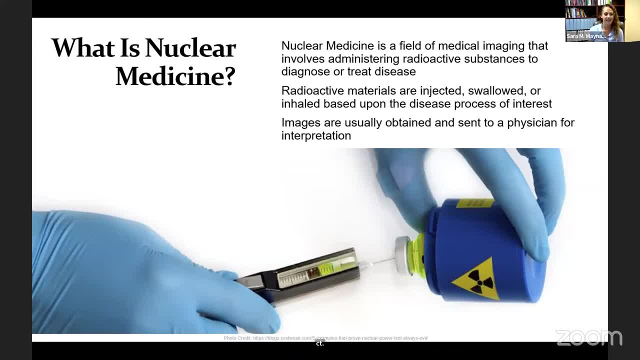 Many of you may be wondering what is nuclear medicine? When I was an undergrad at ODU, if you asked me what nuclear medicine was, I had no idea. So nuclear medicine is a field of medical imaging. It involves administering radioactive substances to patients to diagnose. 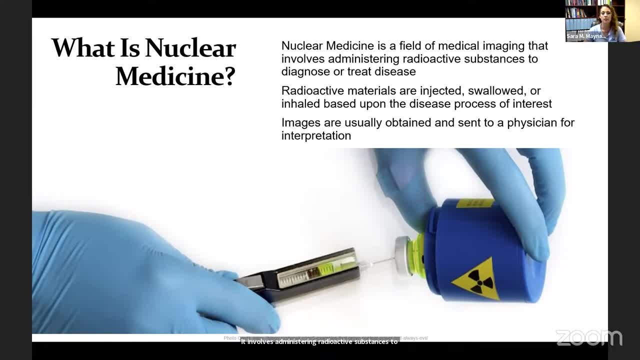 and sometimes to treat diseases. So these radioactive materials that we give to patients, we majority of the time will inject them, Depending on what body system we're looking at. they can also be swallowed by the patient or inhaled, based on what disease process we're looking at. We do a really interesting study. 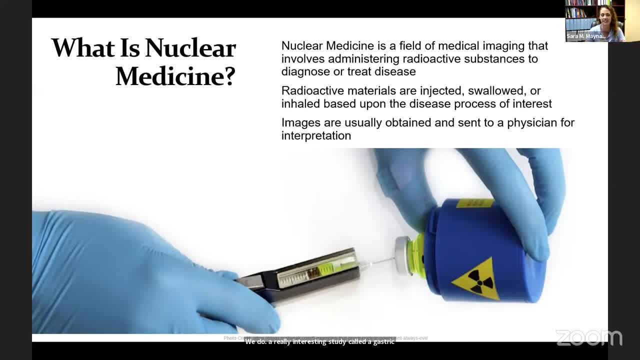 called a gastric emptying study, where we mix in radioactive materials with eggs. the patient eats them and we watch to see how fast or slow their stomach digests the eggs. After we administer the radioactive materials, we usually take images and send them to a physician. 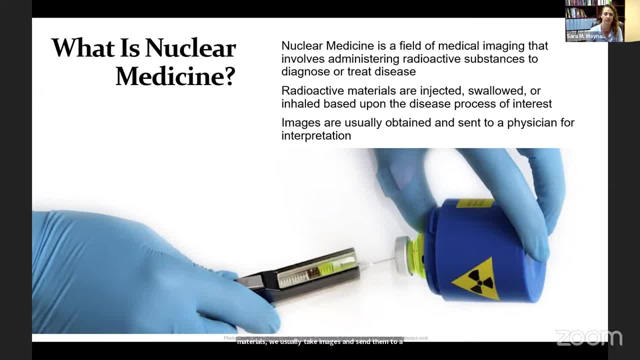 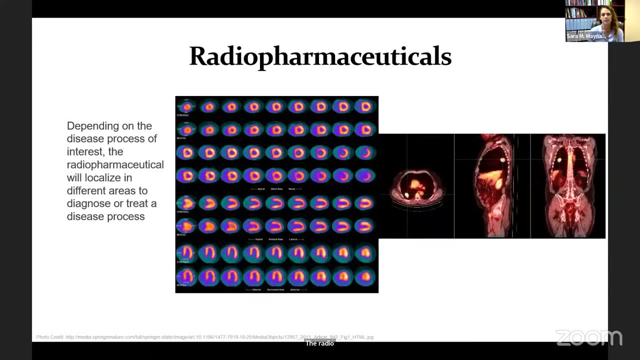 called the doctor. So we take the images and we send them to a physician called the doctor. So we take the images and we send them to a physician called a radiologist for interpretation. The radioactive material that we administer to the patient is called a radiopharmaceutical. 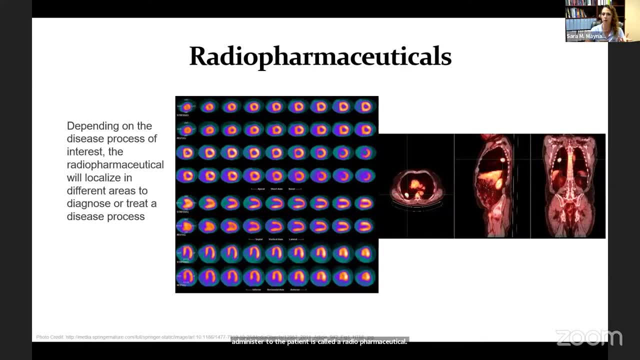 So it's a radioactive isotope, which is the part that we're actually detecting, combined with the pharmaceutical, So that'll make it go to a different place in the body. If we're looking at the gastric system, if we're looking at the heart, we give different 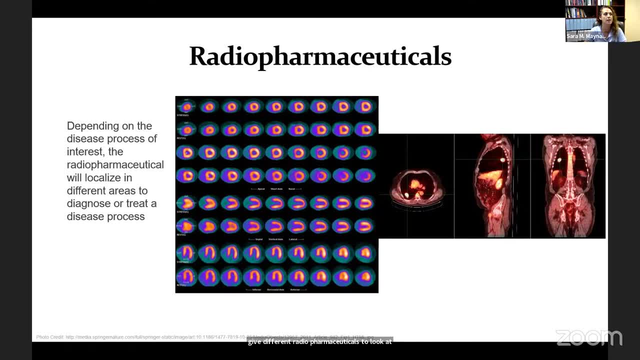 radiopharmaceuticals to look at different body processes. So depending on the disease process of interest, our radiopharmaceutical will localize in different areas to diagnose or treat a disease process. So I'm going to talk about these in a little more detail later in the presentation. 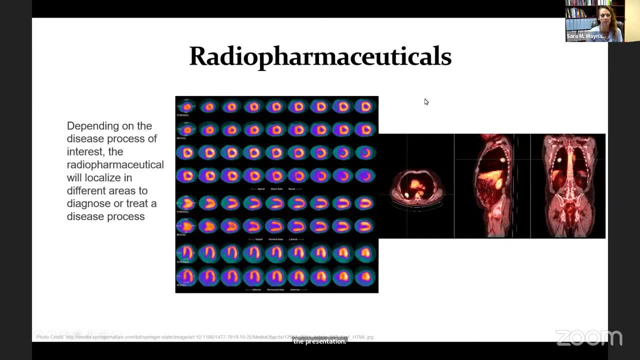 But this one on the left here you see, with all the colorful circles. this is a really common test that we do called a nuclear stress test. So we actually that radioactive material and it shows us the blood flow distribution to the heart. We're trying 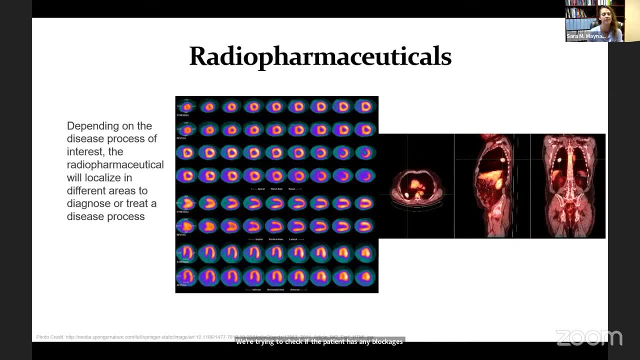 to check if the patient has any blockages in the heart muscle. This other one is really the up-and-coming technology in our field. It's called PET-CT. We administer a radioactive sugar to the patient. Certain types of cancer will take up more sugar than the surrounding area and show up. 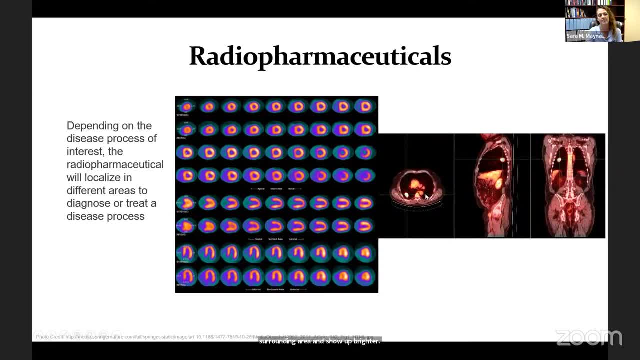 brighter. So you see some green crosshairs here over a really bright section. So that is actually a cancer in the lung. Certain other types of imaging rely on changes in the structure to relay disease processes. That's what's so interesting about nuclear medicine and PET-CT. 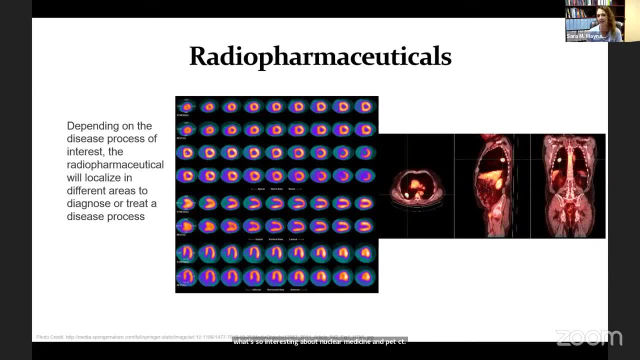 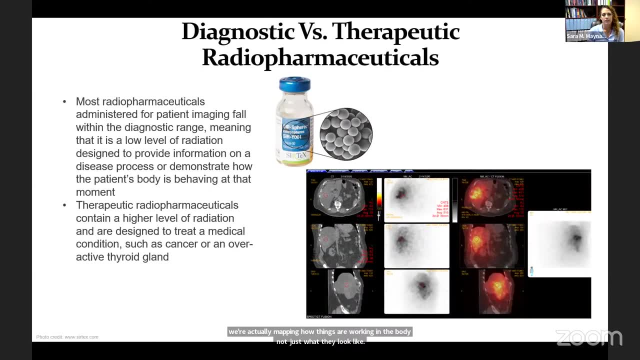 is we're actually mapping how things are working in the body, not just what they look like. So we have different radiopharmaceuticals for different purposes. We have diagnostic versus therapeutic radiopharmaceuticals, So most radiopharmaceuticals that we administer. 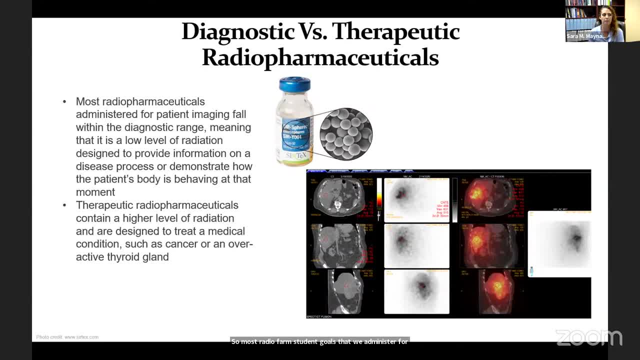 for patients fall in the diagnostic range. That means it's a low level of radiation and we're just trying to provide information on how the body is behaving or how that disease process is behaving at that present moment. We want to essentially make sure that we're. 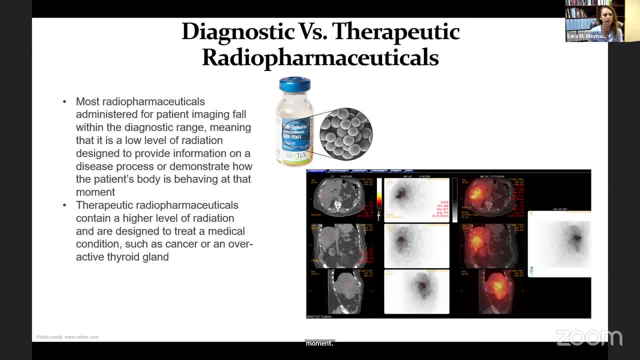 mapping what's going on in the patient's body. Therapeutic radiopharmaceuticals contain a higher level of radiation, So they're designed to treat a medical condition such as cancer or an overactive thyroid gland- A really interesting procedure that I get to be a part of a lot when 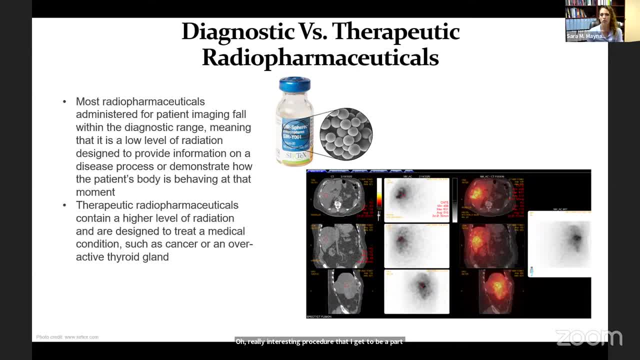 I work at Sentara, Norfolk General Hospital. it's called Yttrium-90 microspheres, So they're tiny microscopic spheres that are, in a liquid suspension, designed to treat liver cancers. So an interventional radiologist will go in through one of the liver arteries. 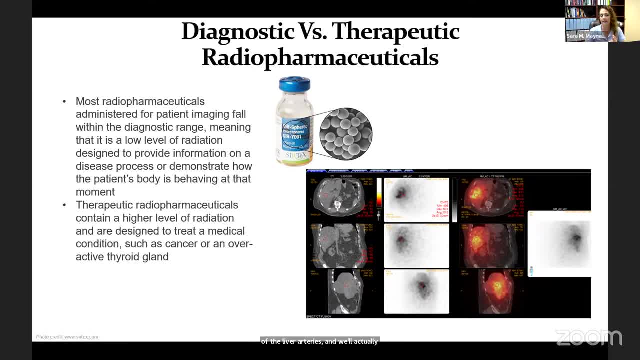 and we'll actually administer these radioactive spheres into the liver tumor. The whole goal of this procedure is to try to treat that liver tumor and preserve as much of the healthy tissue around it as possible. External biopsy is a very common procedure that we use to treat liver cancer. 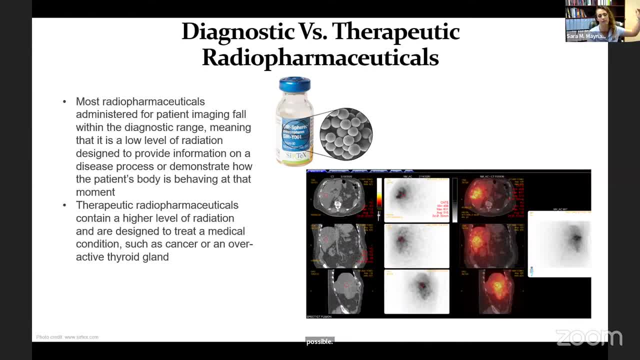 The whole goal is to try to treat the liver tumor and preserve as much of the healthy tissue around it as possible. External biopsy is a very common procedure that we use to treat liver cancer, So we end up inadvertently hitting a lot of healthy tissue on the way. So these targeted radiopharmaceutical 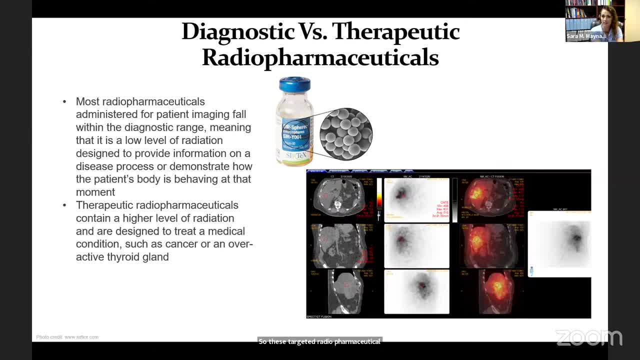 therapies are designed to kill that cancerous tissue and preserve as much of the healthy tissue as possible. So you'll see on the slide here this is actually an image after we administer the Yttrium-90 spheres. So this is a picture of the Yttrium-90 microspheres And this is a picture of 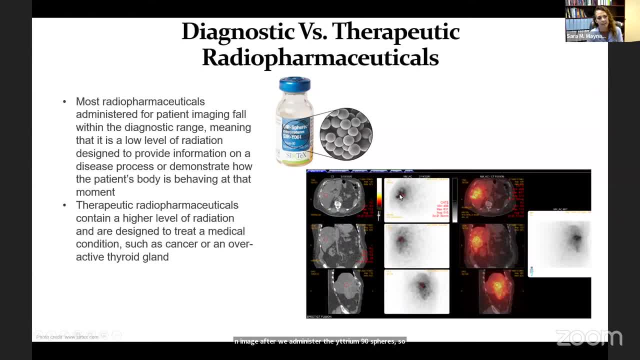 So that really bright concentrated area near that red circle, that's actually where those spheres were delivered. We do a low dose CT scan and we fuse the two. That way afterwards the health physicist and the radiation oncologist can actually track: did we hit as much as we wanted to, how much dose got where and how much of the dose got to the healthy tissue unintentionally? 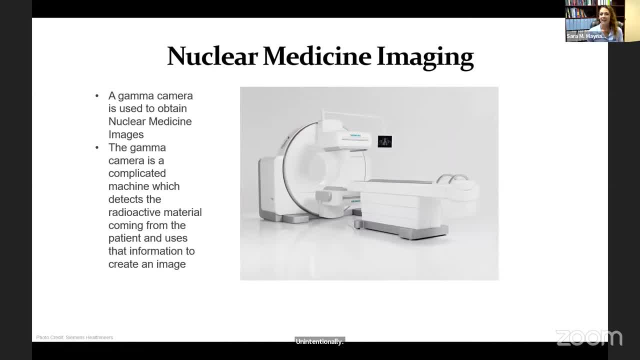 So you may be wondering how we get these fancy images. So some of you may have had a CT scan, an x-ray, an MRI. Our instrument is a little bit different. for nuclear medicine imaging We use an instrument called a gamma camera. 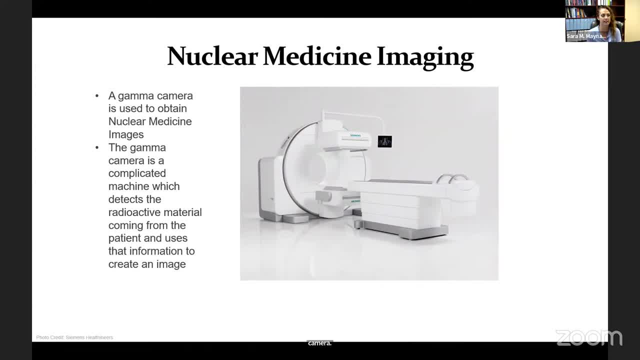 This is a complicated machine which detects the radioactive material coming from the patient and uses that information to create an image. So, as you'll see here, this is this rectangular structure- here Inside there is a crystal So that detects that gamma ray, converts it to a usable electronic signal for the computer. 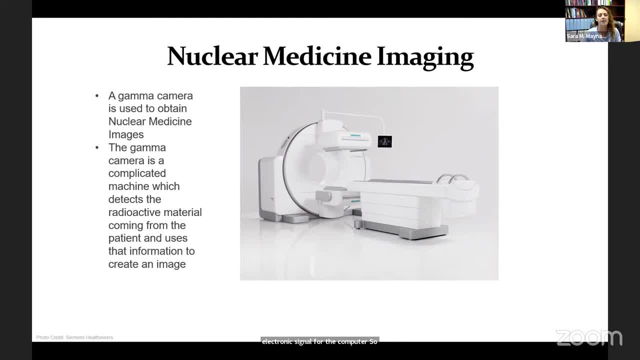 So we can actually map the patient images. So this particular camera has two crystals here. So it's essentially we can get a picture from the top and the bottom at the same time, But depending on what body system we're looking at, we can rotate them 360 degrees around the patient or configure them in different ways to look at different parts of the body. 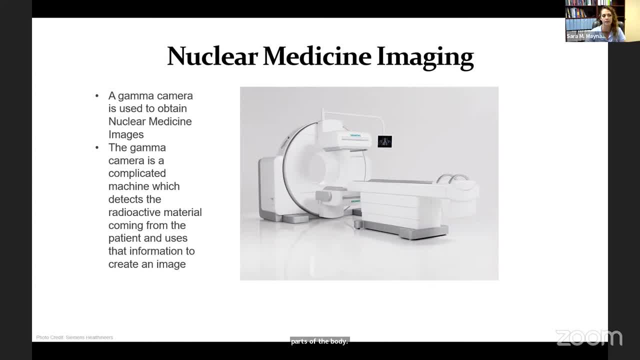 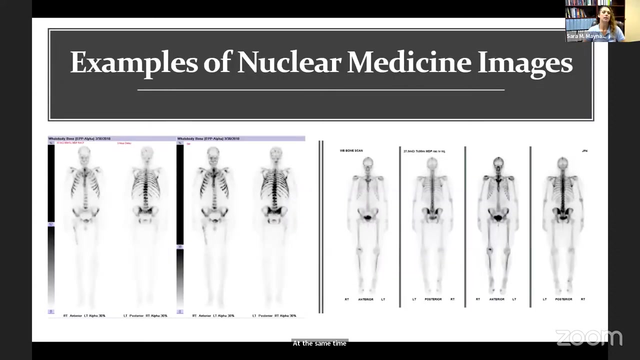 Most modern nuclear medicine imaging systems are also combined with a CT scanner, which is that circular structure on the back there, So we can fuse our images with the CT images and get really good structural and functional information at the same time. So some examples of nuclear medicine images. 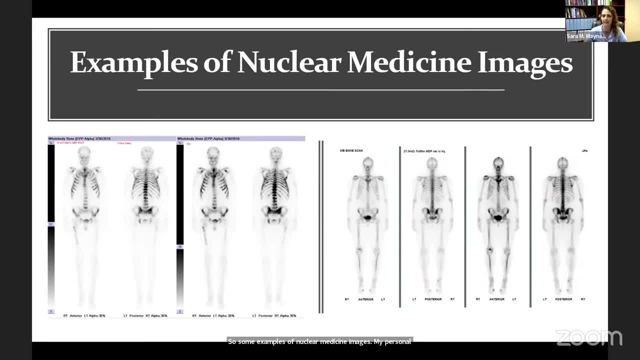 My personal favorite is the nuclear medicine bone scan. We do this for a variety of different reasons, but most often to see if cancer has spread to the patient's bones. So what's different between this and an X-ray? we actually inject the radioactive material into a vein in the arm or hand. 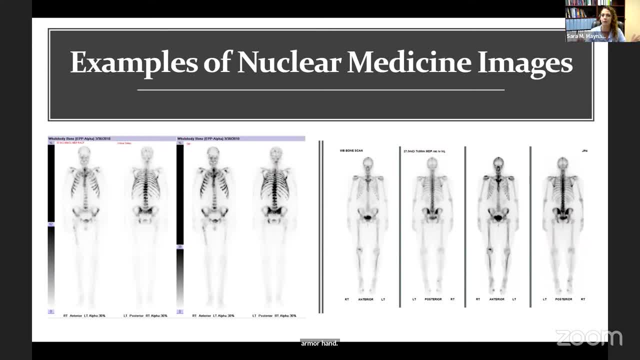 We give it three hours to circulate through the body And get absorbed by the bones. What this radioactive imaging material is showing us is where the bones are rebuilding themselves. So if the patients recently had surgery, they've recently had a fracture. there is some bone remodeling. that goes on. 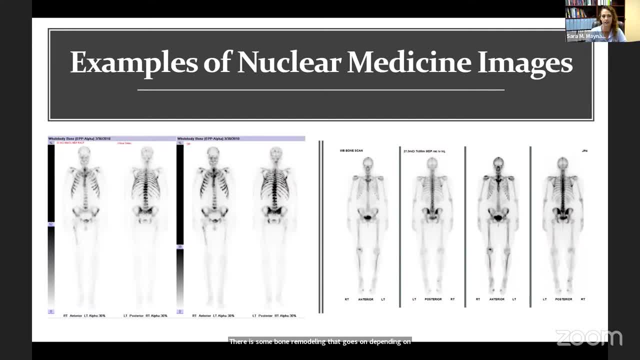 Depending on the pattern of the bone remodeling, the physician can try to determine what disease process is occurring. So this one you see on the right side here, this is a relatively normal bone. We will see the bones. We also see the kidneys and the bladder, because our picture material breaks down and is excreted through the urine. 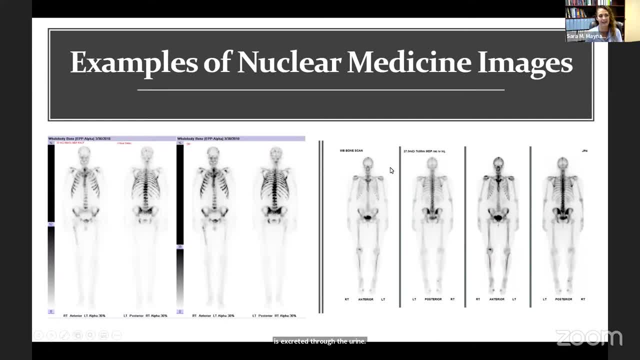 So it looks pretty symmetrical. What we want to see is a nice even distribution on the right and the left side. So this one is from the front, This one is from the back. We also see that bright spot in the pelvis there. 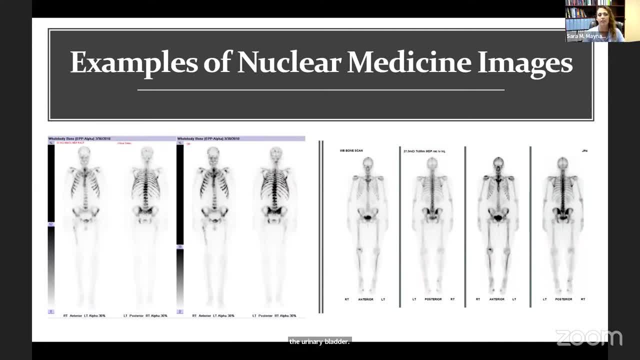 That's the urinary bladder. So overall, things look pretty similar, Pretty symmetrical. On the other hand, this set of images on the left: this shows widespread cancer in the bones. So this is a. I believe this one was a lung cancer that has spread to the bones. 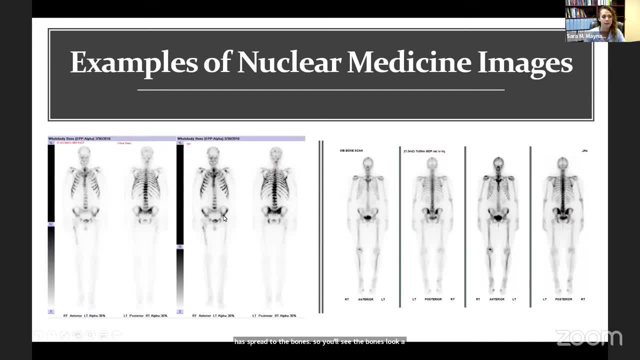 So you'll see the bones look a little modeled. There's some brighter spots all throughout this part of the skeleton: in the skull, in the ribs, the spine, the hips and in the upper femurs. So this one shows. This is one of my favorite studies to do, because I could do a bone scan on every single person in this webinar and they would all look completely different from each other. 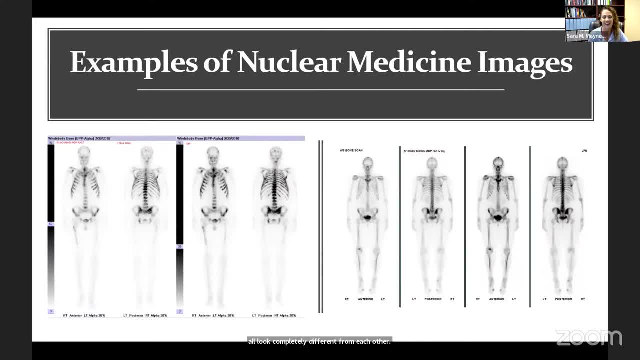 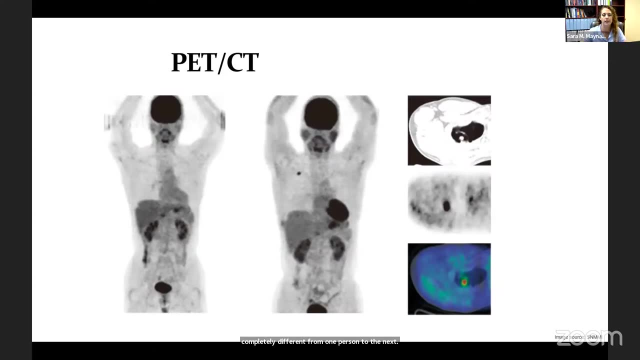 All of our bodies are just built in such different ways, So it's so fascinating. Every day you can have a list of the same studies and it'll look completely different from one person to the next. So another really exciting change to technology recently is positron emission tomography fused with a CT scan or computed tomography. 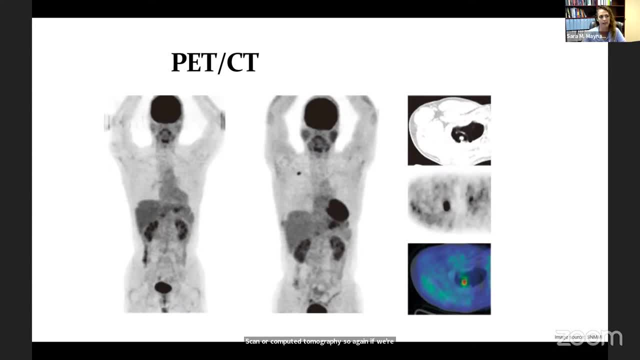 So, again, if we're doing it for cancer screening purposes, we administer a radioactive sugar. Certain cancers will take up more sugar than the surrounding area. So this one, for example. this patient had a CT scan. They saw a little lump in the lungs, but it's difficult to determine if that lump has cancer in it or not just by seeing that it exists. 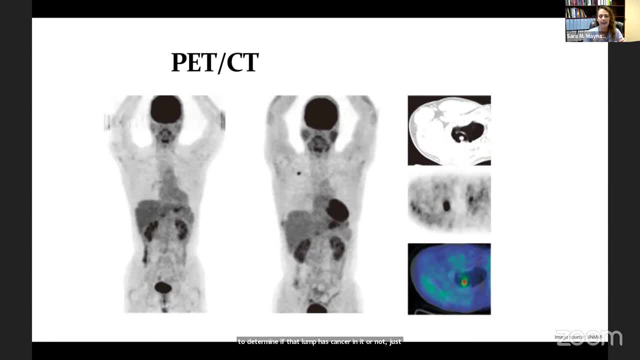 So where they were referred for a PET-CT study. if it lights up brighter on the images, that does mean that there's cancer in that area. So this set of images is normal because there are different structures in our body that take up a lot of sugar. 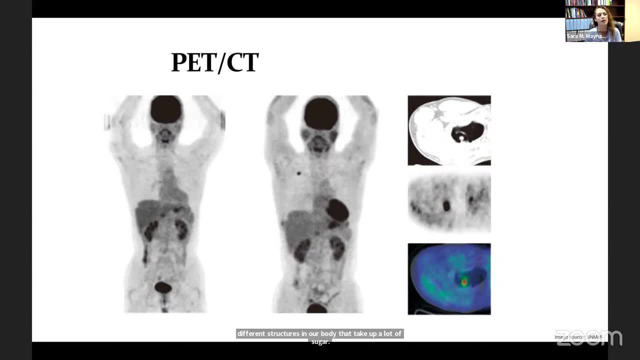 Our heart requires a lot of sugar, Our brains, Our liver a little bit, And then again the urinary system as we break down that picture material and excrete it out of the body. So this one here is relatively normal. This one here, this bright spot in the lungs, indicates a lung cancer. 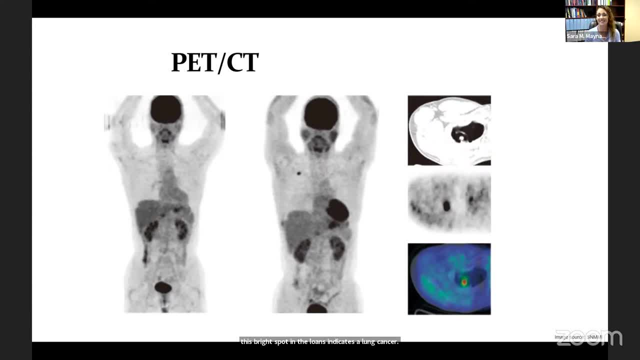 So the field of PET-CT is really exploding. Almost daily they're coming out with different radiopharmaceuticals for different purposes. We have some really exciting things going on right now with prostate cancer. We have some breakthrough technologies that are giving us images that we've never seen before and are really helping us treat these patients better and identify areas of cancer that we've never been able to see before. 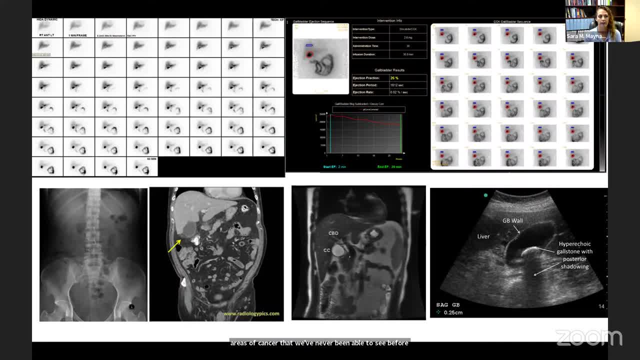 So just an illustration of how nuclear medicine shows us how things are working in the body as compared to other imaging modalities. So the first one here. I'm sure almost everybody knows Everybody on this webinar has seen or maybe had an x-ray before. 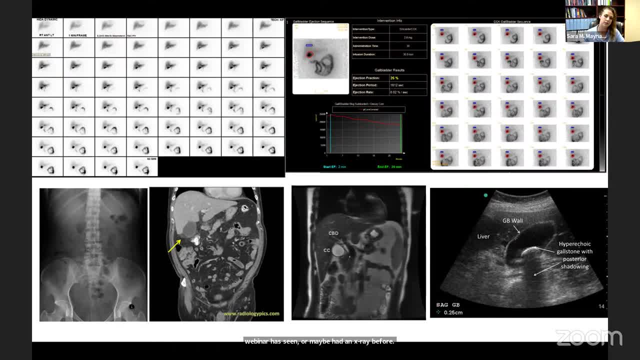 X-rays are inexpensive, They're easy to obtain. They do use a little bit of radiation, but the images that they generate are not amazing. So it's very difficult to see the abdominal structures in this x-ray here. So that's where CT comes into play. 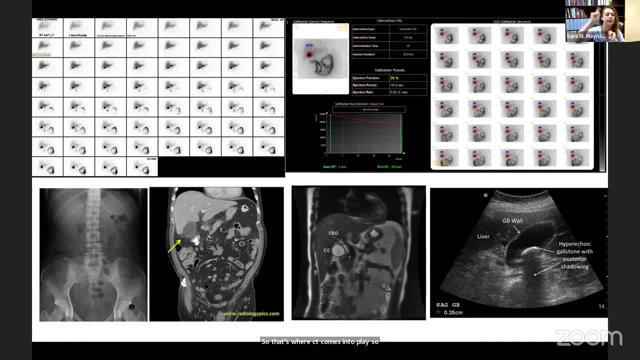 So CT actually rotates an x-ray beam 360 degrees around the patient And it gives us 360.. images of what's going on in the body. So the images are really great for showing the structure, but it's a lot of radiation exposure to the patient. 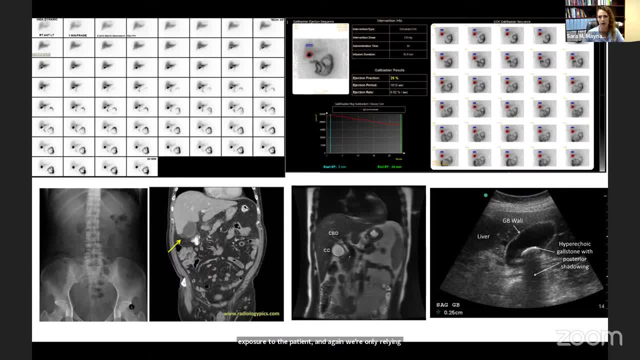 And again we're only relying on changes in the structure of the body to convey disease processes. So for this specific patient example, this is a gallbladder study. So your gallbladder is a small organ in your abdomen. It squeezes bile to help you digest fat. I'm a huge fan of Taco Bell, So every time I eat Taco Bell, my gallbladder is working extra hard to squeeze that bile into my intestines to help me digest fat. If your gallbladder is not working properly, however, when you try to have that Taco Bell experience, you can have some abdominal pain, nausea, vomiting as your body struggles to digest that fatty food. 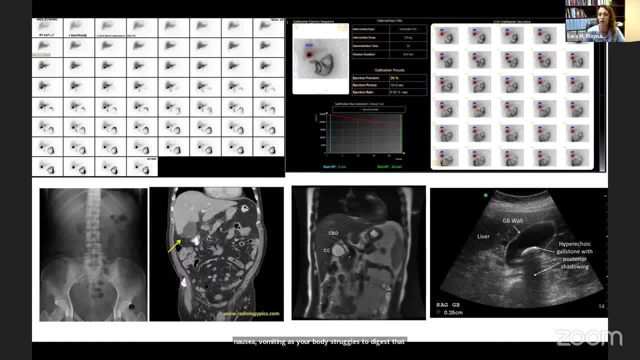 So some indications that your gallbladder may not be good are stones within the gallbladder or fluid around. So that could indicate that your gallbladder is not functioning the way it should, but doesn't necessarily mean your gallbladder is not functioning properly. 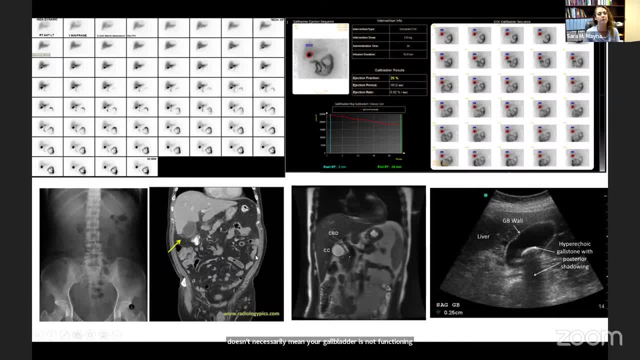 So on the CT scan here the arrow is pointing to some fluid around the patient's gallbladder. Could mean it's not functioning, but not necessarily So. this one here is an MRI or magnetic resonance imaging, So it uses magnets again to generate images of the structures within the patient's body. 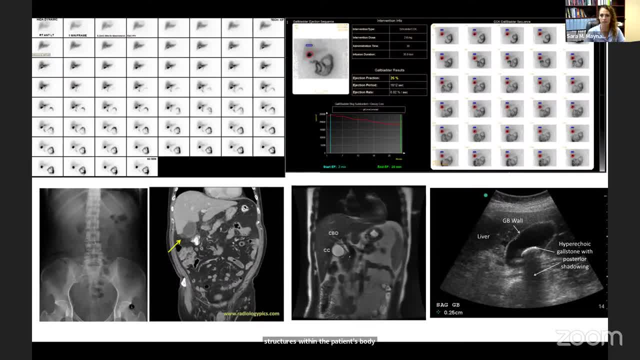 The images are beautiful. However, we're still relying on changes in the structure to convey disease processes in the body. This final one here, this is an ultrasound- Again, no radiation exposure inexpensive to obtain, But the images are only showing us what the structure looks like. 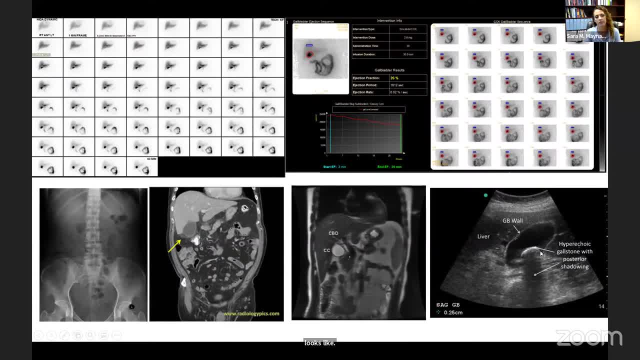 So this patient here, this is the gallbladder, this little circle. there's some stone shown within the gallbladder. Just because you have stones in the gallbladder doesn't mean it's affecting the function at all. So that's where nuclear medicine comes in. 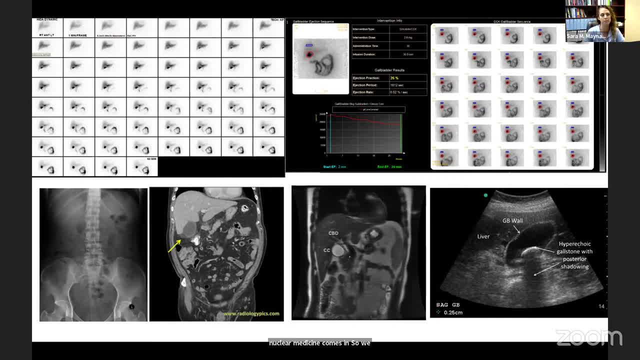 So we administer a radiopharmaceutical that mimics bile. So for the first hour of imaging, we're actually watching the liver create the bile. It goes through the ducts into the gallbladder, which shows up as this brain. It goes through the gallbladder, which shows up as this brain. 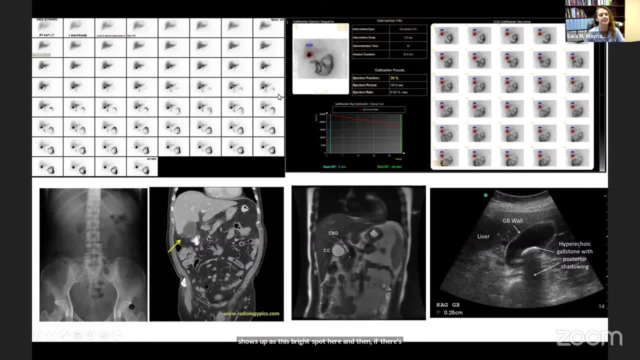 And then, if there's no blockages, it'll empty into the intestines to help you digest that fatty food. If there's no blockages in the pathway leading into or out of the gallbladder, we proceed to the second part of the test. 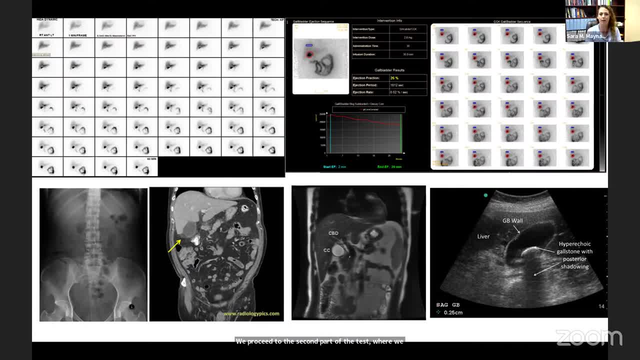 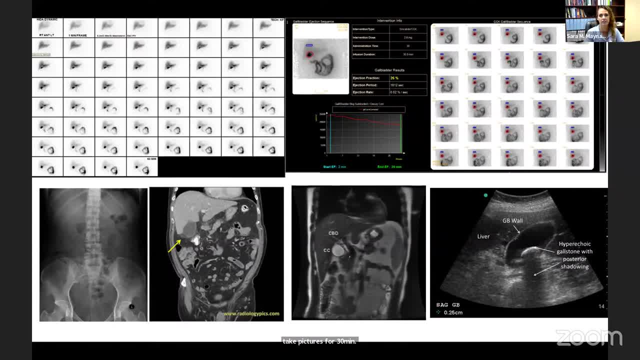 We'll take pictures for 30 minutes. We'll run them like a video. At the end we actually can do some calculations to see how well or not well the gallbladder is squeezing to help you digest that fatty food. So my role as the technologist is to look at the images. 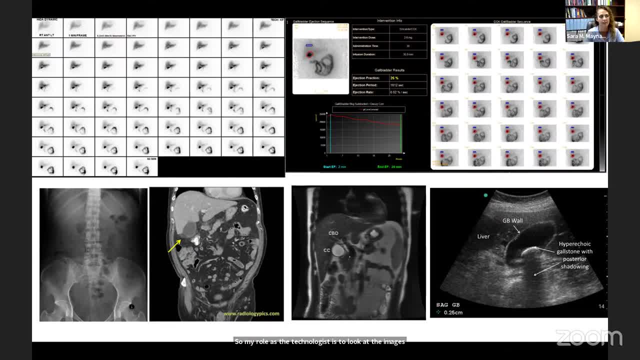 I have to identify. yes, I saw the gallbladder, I saw the liver, I saw the intestines. That pathway's open. I can give that fatty medication and watch the gallbladder squeeze for 30 minutes And then we can do the next step. 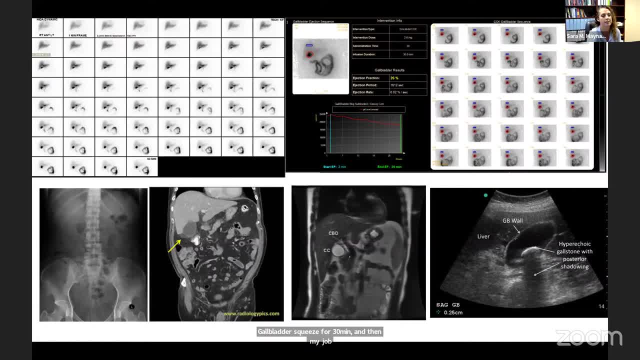 And then my job afterwards is to do the calculations. So this patient's gallbladder is not functioning where it should be. Normal is above 35%. Their gallbladder is only squeezing 26%, So they're probably due to have their gallbladder removed very soon. 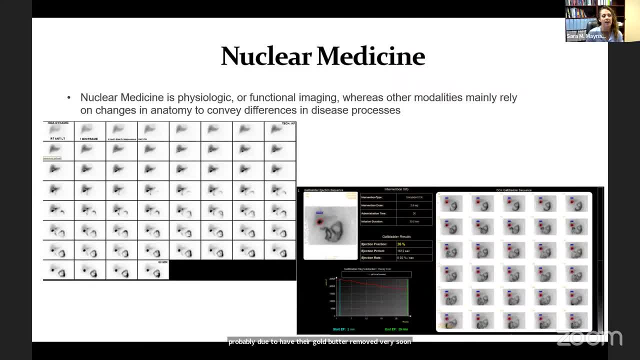 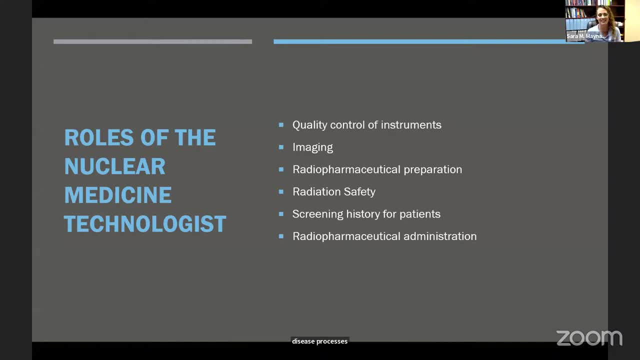 So, in summary, nuclear medicine is physiologic or functional imaging, whereas other imaging modalities rely on the gallbladder, They rely on changes in the anatomy to convey differences in disease processes. So what does a nuclear medicine technologist do? So our roles are quality control of all the instruments. 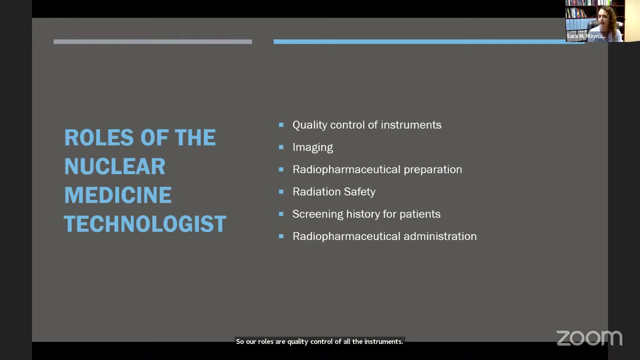 It is very important that we're giving a safe amount of radioactive material to patients. Too much radiation can be harmful, So it's very important that we're in a precise range, that we have instruments that also check after. at the end of the day, 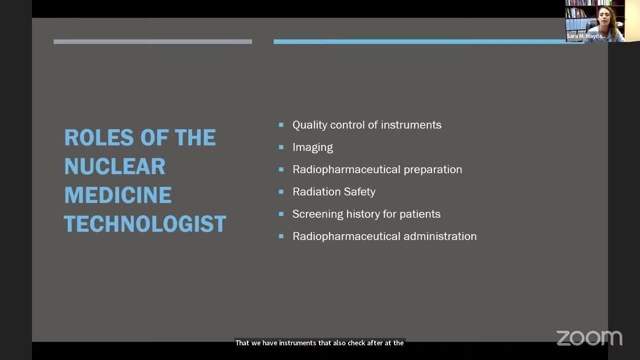 that we didn't leave any radioactive contamination anywhere, that our image machines are working properly and that we're keeping both our patients, staff and those outside of the department safe. Another role of ours is imaging. We have to obtain the images. 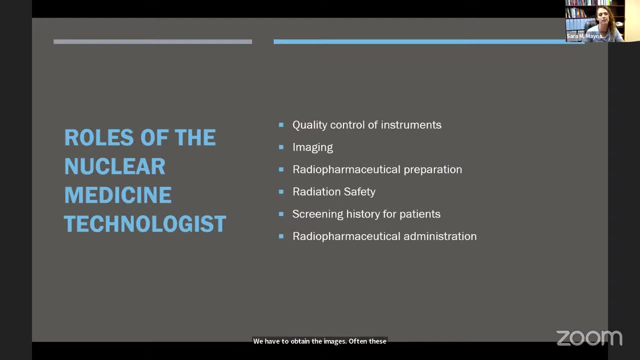 Often these patients are very ill. They're not feeling well. So our job is to get the best possible image for each patient every time, And sometimes it involves a great degree of creativity. Not every patient is going to be 30 years old and able to walk. 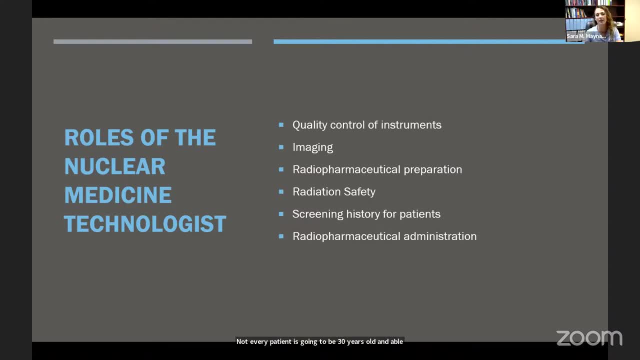 able to talk to you, able to understand you. So sometimes you have to get creative to get the images that you need to get that patient the help that they need. Another part of our role is radiopharmaceutical preparation. We're responsible for administering these radioactive materials. 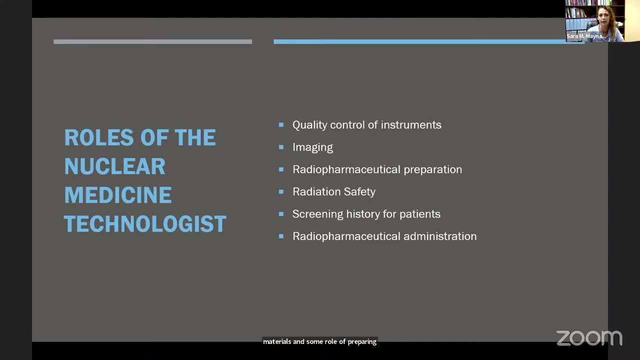 and some role of preparing them. It's very important that we understand the patient's history, any medications that could affect the radiopharmaceuticals and how they're delivered to certain areas of the body, and that we're very, very good at injecting these radioactive materials. 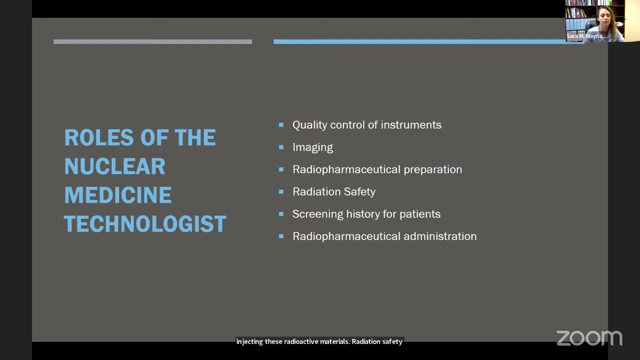 Radiation safety is very important for us, for our patients and for those in the surrounding area. And screening: we want to make sure we're studying the function of the body. There's so many things that can affect the function of our radiopharmaceuticals. 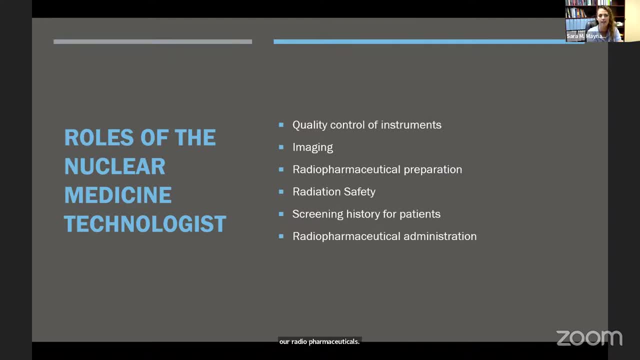 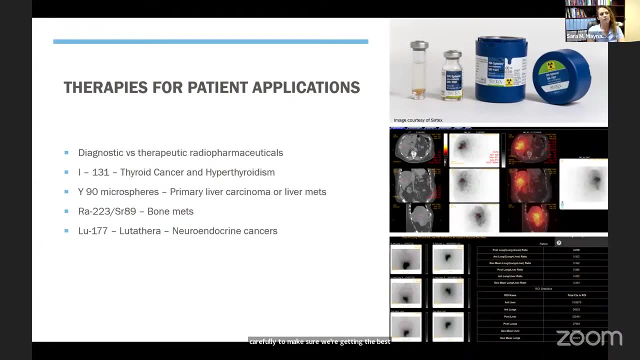 So it's really important for us to screen our patients carefully to make sure we're getting the best possible tests every time. So one thing that prospective students are always really interested in and is pretty rewarding to be a part of as a nuclear medicine technologist is therapies. 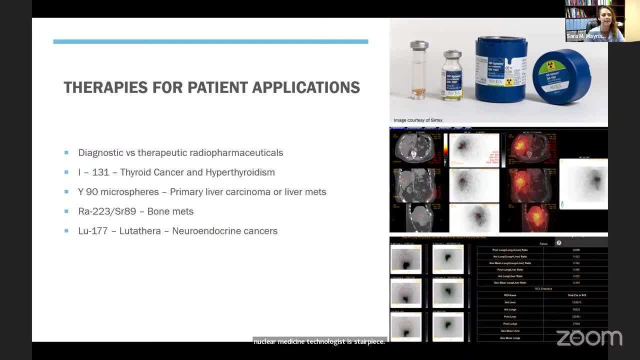 So some of the therapies that we are involved with. so again diagnoses. So some of the therapies that we are involved with. so again diagnoses. So some of the therapies that we are involved with. so again diagnoses. So for diagnostic radiopharmaceuticals. 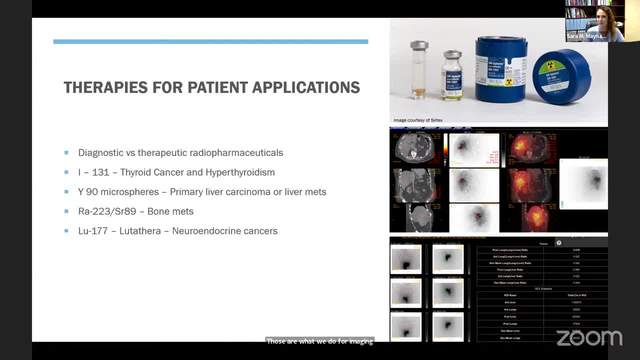 those are what we do for imaging how different body systems are working. Therapeutic radiopharmaceuticals are actually trying to destroy some tissue, So they're a higher range of radioactive materials and they require more radiation safety precautions as well. So some examples that you may or may not have heard of. 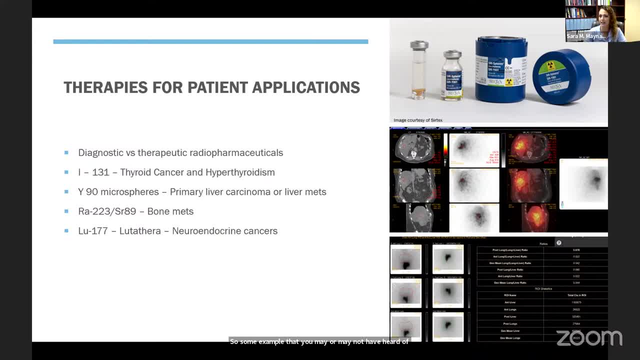 are iodine-131, usually for thyroid cancer or for overactive thyroid, or for overactive thyroid to try to destroy some of the thyroid cells. As I discussed the Y90 microspheres for primary liver cancer or cancer from somewhere else that has spread to the liver. So these are the ones. 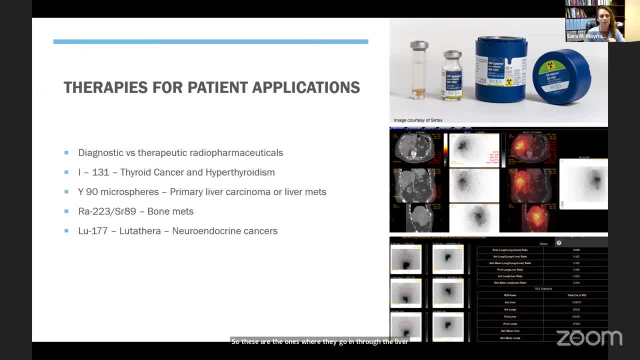 where they go in through the liver artery and they administer the microscopic spheres to treat that liver cancer. We also have some other bone cancer treatments, So radium-223 and strontium-89 and a pretty new exciting one for neuroendocrine carcinoma called Lutathera-177.. 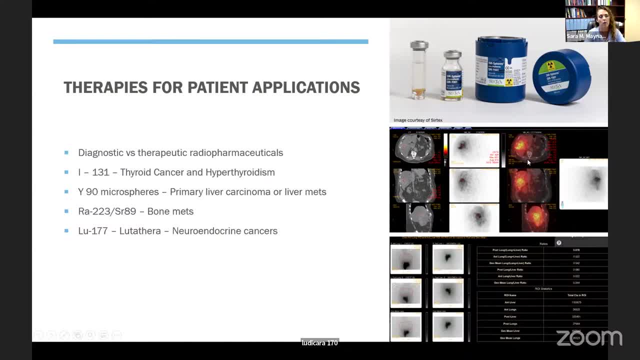 So this here is more examples of the Y90 imaging. So this is after the therapy. We also do some imaging before the therapy. as a little tester, We give a diagnostic radiopharmaceutical that has a similar particle size. We actually map out how much goes to the 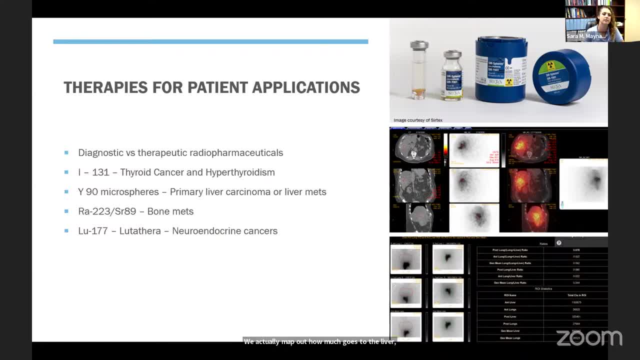 liver tumor. how much goes to the lungs to make sure it's even safe to treat this patient? We don't want our whole dose of the microscopic spheres to go to the patient's lungs and irradiate the patient's lungs. So we do a tester procedure before we administer. 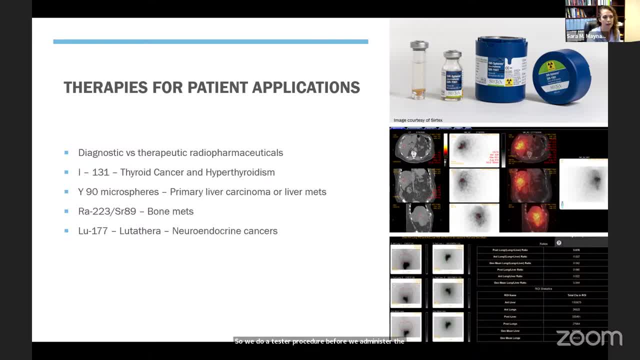 the therapeutic pharmaceutical. So part of my job is calculating how much went to the lungs and how much went to the liver. So we do a tester procedure before we administer the therapeutic pharmaceutical. So part of my job is calculating how much went to the lungs and how much. 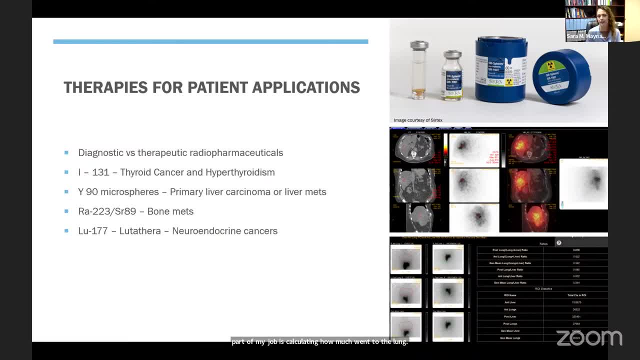 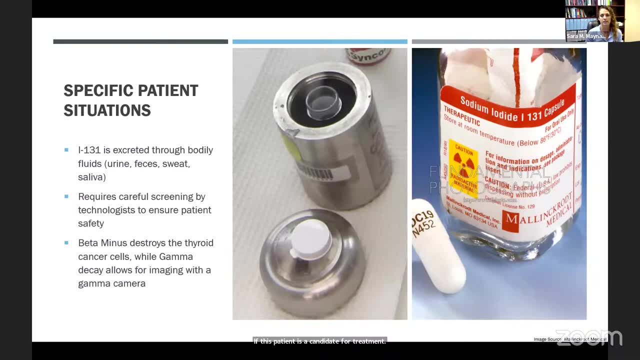 went to the liver, So the physician can decide if this patient is a candidate for treatment. So I wanted to share a couple of interesting patient case studies. So one is a iodine-131 thyroid therapy. So iodine-131 is a therapeutic radiopharmaceutical, So it's a higher level of radiation. It's usually to treat ovarian cancer. So iodine-131 is a therapeutic radiopharmaceutical. It's usually to treat ovarian cancer. So iodine-131 is a therapeutic radiopharmaceutical. So it's a higher level of radiation. It's usually to treat ovarian cancer. So iodine-131 is a therapeutic radiopharmaceutical. 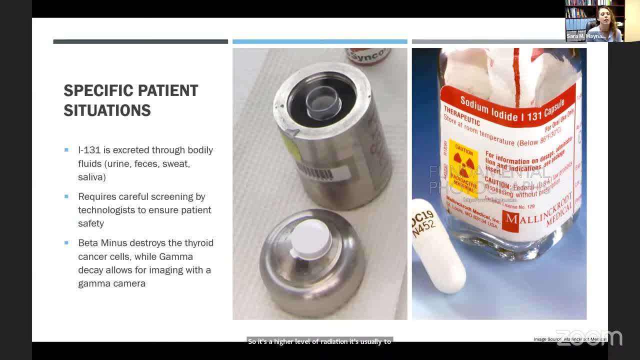 It's usually to treat ovarian cancer. So iodine-131 is a therapeutic radiopharmaceutical. So iodine-131 is a. The iodine-131 is broken down and excreted through bodily fluids, so urine, feces, sweat and 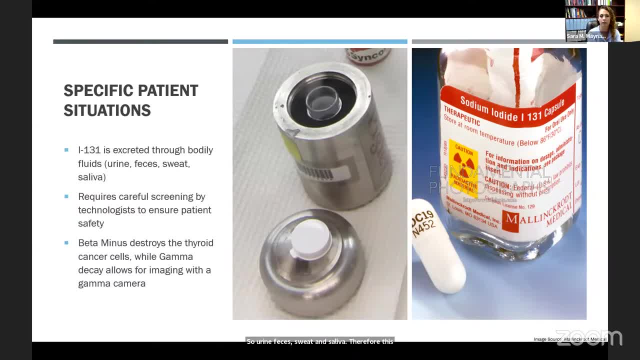 saliva. Therefore, this requires very careful screening by the nuclear medicine technologists to ensure patient safety. These patients, depending on the level of dose that they're getting, will be radioactive anywhere from several days to several weeks, Depending on how high of a dose that they're getting. So we have to carefully screen these. 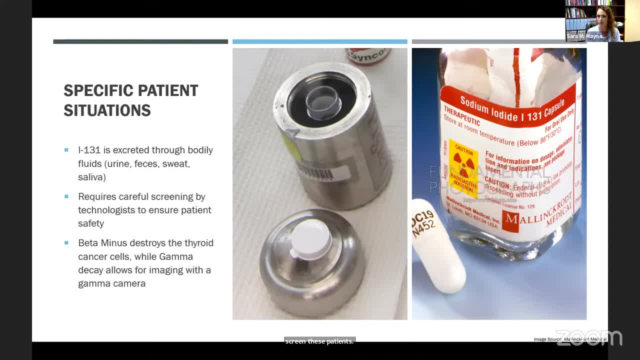 patients. We want to make sure females are not pregnant, as that radioactive material could harm an unborn baby. We want to make sure that it's not a situation where there's no other room for the patient to sleep, While they have a very high level of radiation. 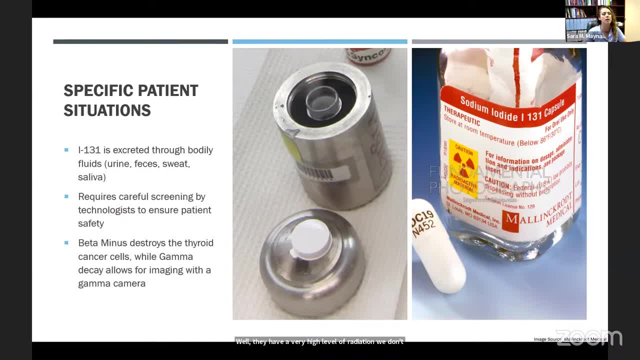 we don't want somebody laying in the bed next to them- That the patient is able to control themselves when they urinate, when they go to the bathroom, because their bodily fluids are radioactive as well. So part of our role is calling these patients personally in advance, making sure that they're even candidates to receive this treatment. 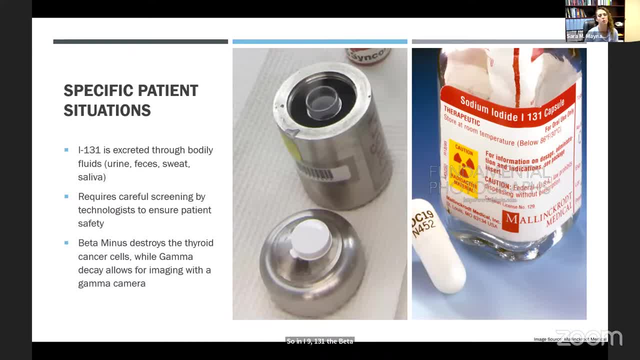 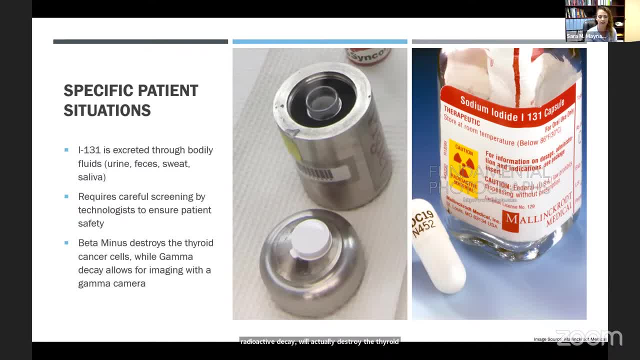 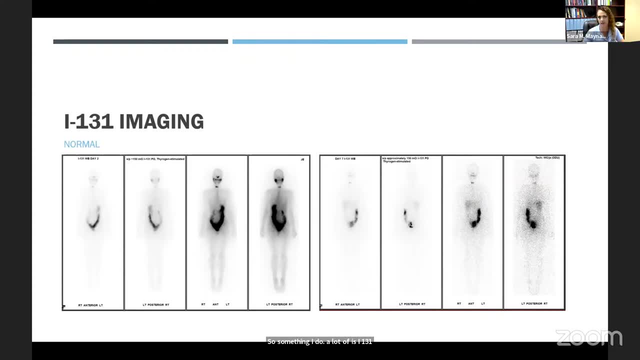 the ability to destroy the thyroid cancer cells. It also emits a gamma ray that allows us for imaging. So something I do a lot of is iodine-131 imaging after a patient has been treated for thyroid cancer, So it's no additional radiation exposure to the patient. 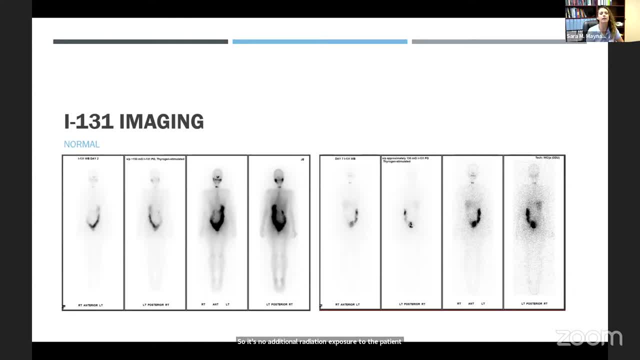 The beta-minus is actually treating the thyroid cancer and we're using the gamma rays to create images and see if we see any thyroid cells outside of where we would expect. So you'll see, this is normal. This patient we imaged usually at two days and at seven days. So the little dots right here. 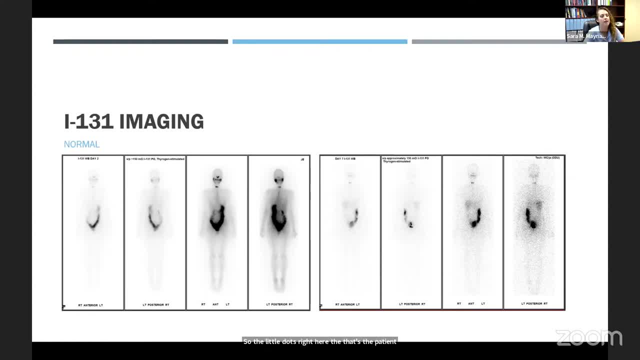 that's the patient's thyroid gland, So that's being treated. We also see the salivary glands. that's normal. We also see it breaking down and going through the GI system and the urinary system, So that is completely normal. But sometimes what makes nuclear medicine and working with patients so? 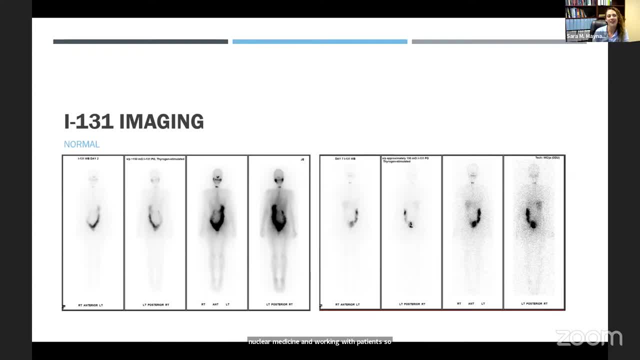 interesting is not every day is normal. So the next one I'm going to share is a patient who came to us for his seven-day post-imaging study and we were all very, very confused. So, again, normal. we see the salivary glands, the thyroid glands, the urinary and the GI system. However, 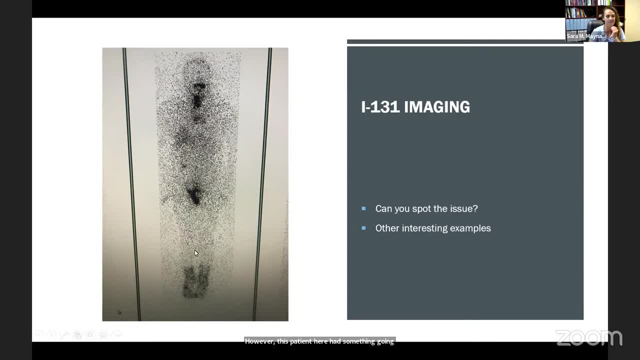 this patient here had something going on with his thyroid gland, So his diabetes was low and he was not feeling well. his blood pressure wasn't his feet, Um. so it turns out- this is a seven day post-therapy study- that radioactive materials excreted through bodily fluids, urine, feces, saliva and sweat, Um, it turns out that this. 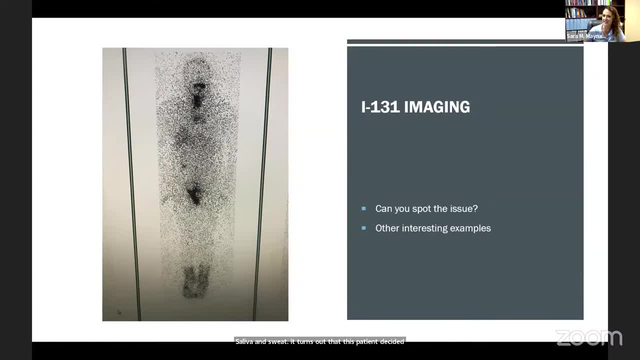 patient decided to wear the same pair of socks for seven days after his treatment without watching them, washing them. Um, so we saw his sweaty socks in the images. So what's really interesting about my job is sometimes we have to think outside of the box, problem solve and get creative about. 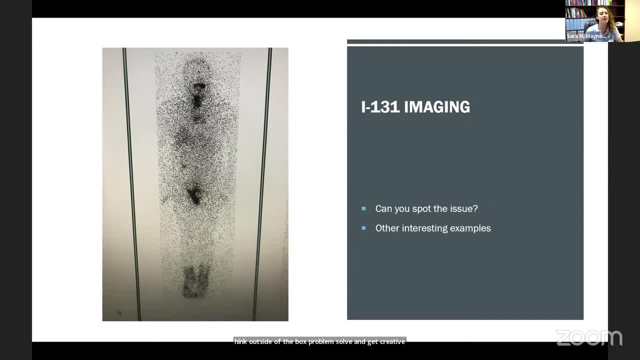 why we're seeing unexpected things in the pictures. Another really interesting one: um, this is pre-COVID, but it was cold and flu season. The patient had a little bit of a runny nose. Um, she actually had a top. 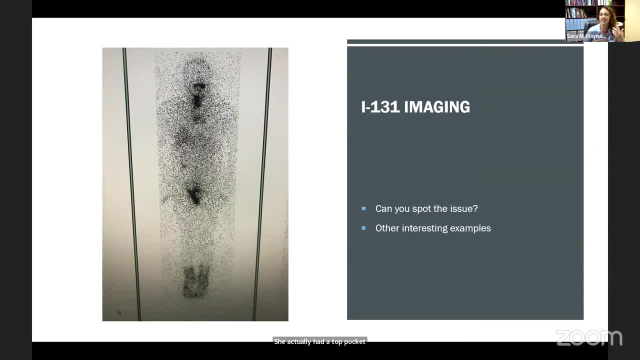 Pocket in her shirt and she had a tissue in her top pocket. We were very worried that we saw some of the thyroid cancer in her lung. So when we rotated the camera a different way, we saw that it was actually resting on top of her body, not in her body. Um so, very interesting problem solving. 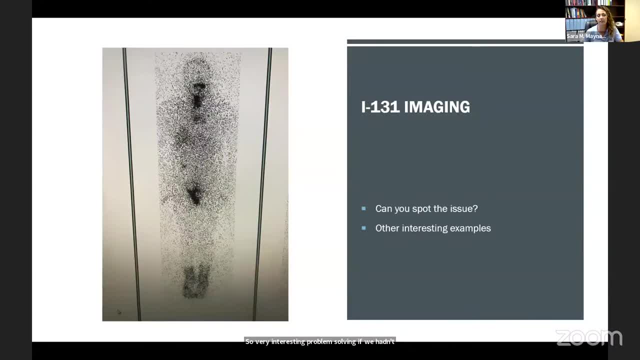 If we hadn't taken that step, she potentially could have been treated for a tumor in her lungs that she didn't have when it was. So that was really just. she had a runny nose. We see the saliva, um, and it was just saliva on her tissue, So that was a pretty crazy one as well. 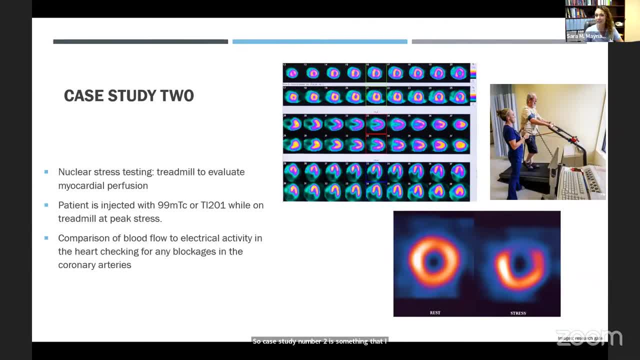 So case study number two is something that I spend the majority of my day in nuclear medicine doing. It's called a nuclear stress test, So it's essentially a before and after picture. We start an IV, We administer the radioactive test, We take some of the radioactive imaging material. 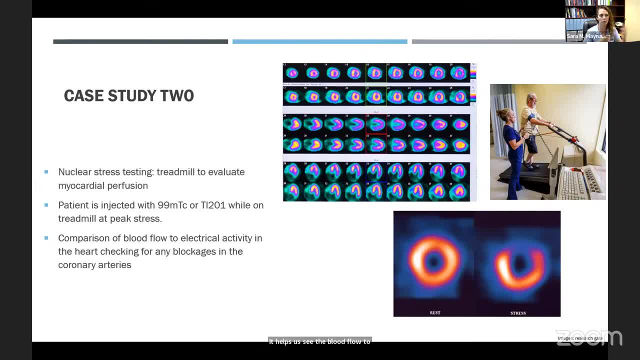 Um, it helps us see the blood flow to the heart muscle. So we take a picture while the patient's heart is at rest and then we stress the heart so they'll walk on the treadmill if they're able to. If not, we'll give them a medication instead that takes the place of walking on the treadmill to stress the heart. 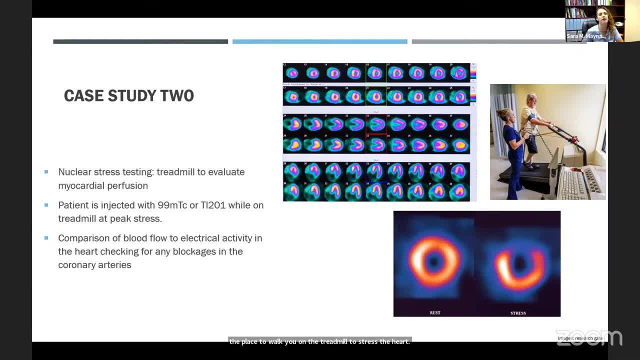 Um, we'll take another set of images after and compare the two. So this first set of images here is nice and normal, is a nice fat squishy donut between rest and stress. What we don't want to see is this bottom. 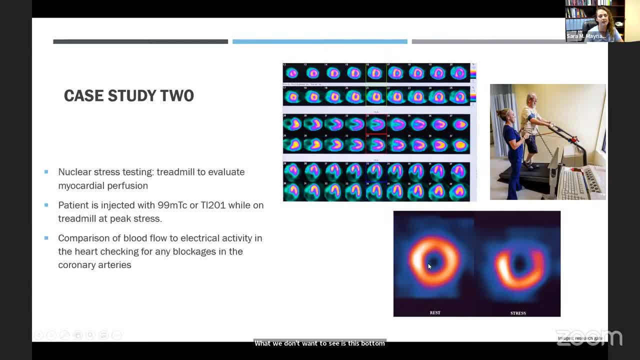 set of images here. So a nice squishy donut in the rest and a bite taken out during the stress. That means that one of those arteries is blocked While the patient's heart is being stressed. the artery is closing off and not delivering as much blood flow as it should to the heart muscle. 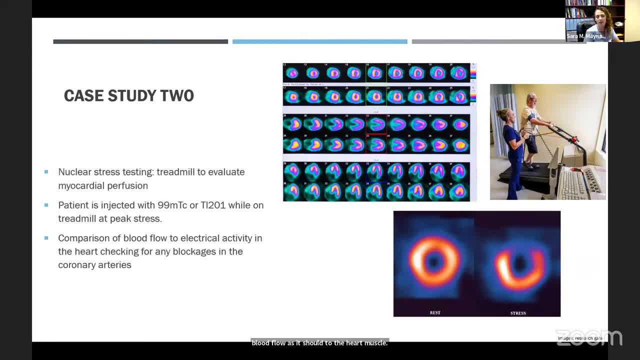 Um, so they might be a candidate to go get a cardiac cap, which is essentially like sticking a straw in the artery to open it back up. Or, if it's bad enough, they may need a bypass surgery. So go around that blocked artery and create a new pathway. So while the patient is being 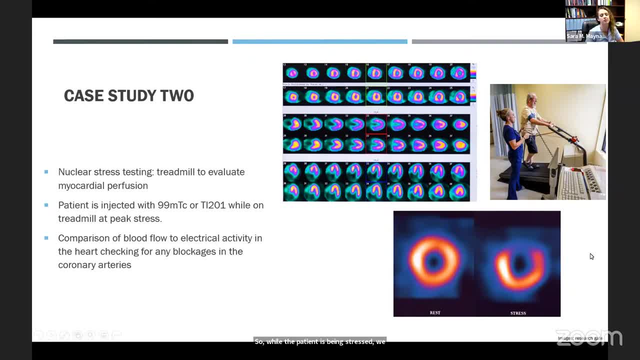 stressed, we compare the electrical activity in the heart to the blood flow images that we obtained, So these are always really, really interesting. Um, it's really fun to look at the blood flow images that we obtain, So these are always really really interesting. 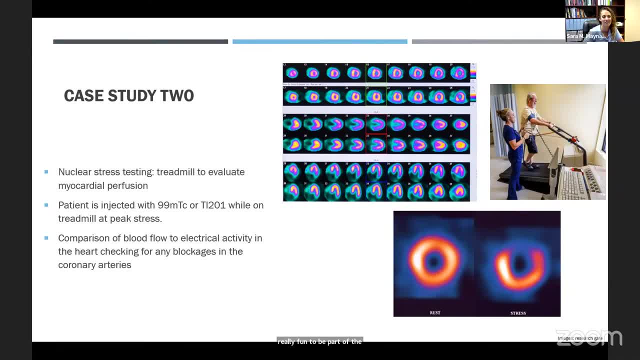 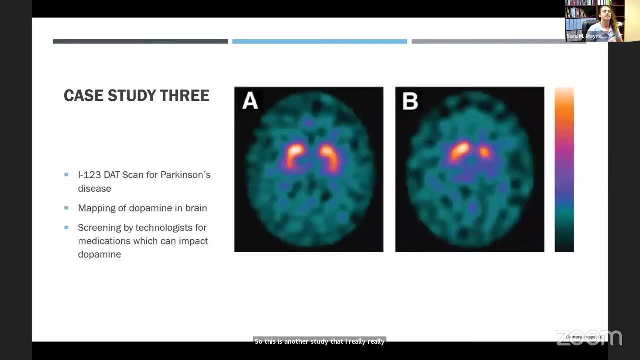 To be part of the interesting things can happen in the stress lab, Um. so this is another study that I really, really enjoy. Um and my final case study here is one study that's really been picking up um in popularity in the last couple of years. it's called I-123 DAT scan. So the 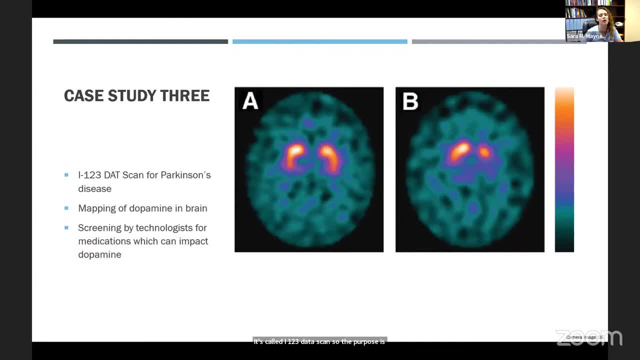 purpose is to diagnose Parkinson's disease. So what we're doing is we're actually mapping the dopamine in the brain. So it's essentially a radioactive cocaine analog that maps the dopamine um deposits in the brain. So patients that have Parkinson's disease have different dopamine. 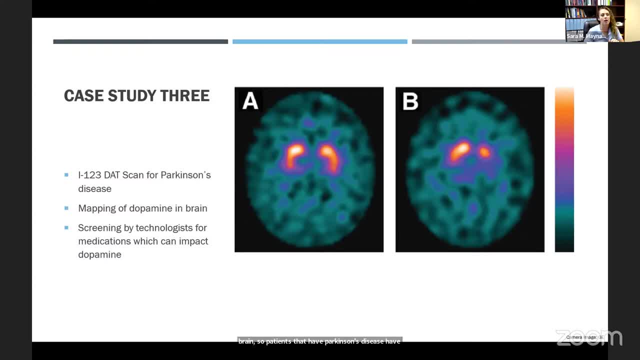 distribution than a normal patient Um. so a really interesting part of being a part of this study is there's about a 10 to 15 page book of medications that can affect the dopamine um distribution In the brain. So we have to screen these patients, make sure that they're off of these medications. 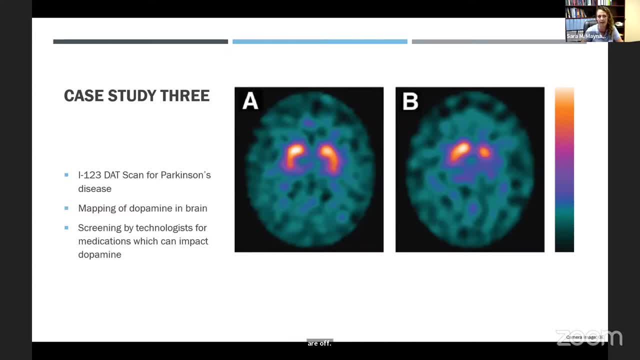 or other substances that can impact the dopamine in the brain. What we want to see is a um, so that looks like a little comma in the brain. So that's normal distribution in the brain. What we don't want to see is it look like a period. So commas are good, period is bad, So that indicates that. 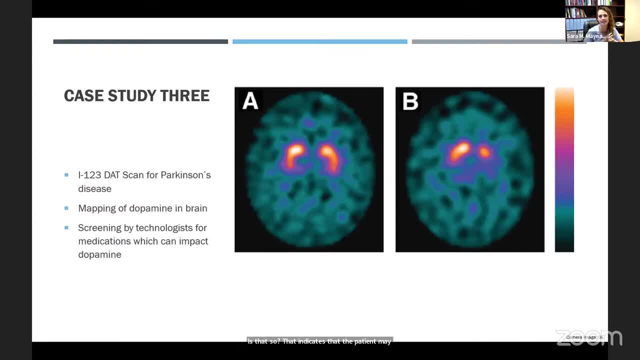 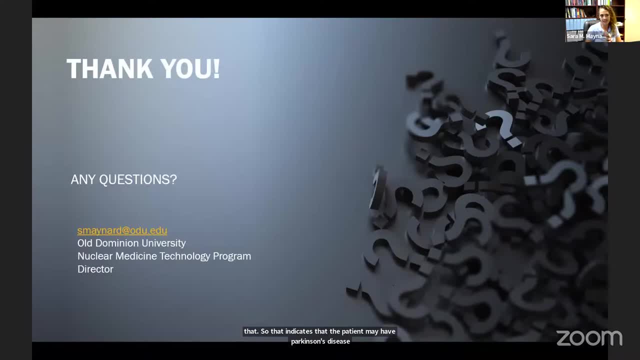 the patient um may have Parkinson's disease, Dr. So this concludes um my presentation and I wanted to open it up to any questions from the participants, Dr. Thank you, Ms Maynard, for talking with us about your clinical work at ODU and Sentara and the use of nuclear physics and medical applications. 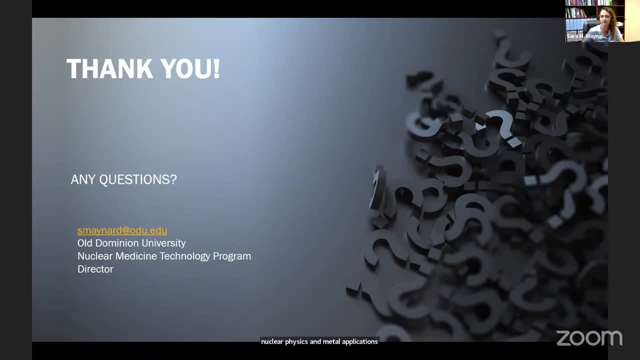 Um, now we're going to take questions from our live audience. As a reminder audience, you can submit your questions in the Q and A box on your Zoom screen and we will answer as many of those as time allows, Dr Um. so one of the questions: earlier you mentioned that some cancers absorb more sugars than the surrounding areas. 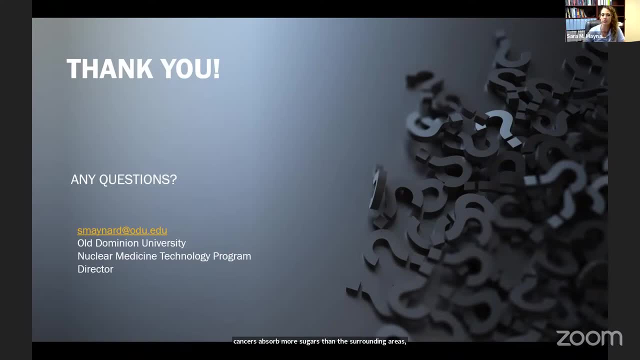 and therefore show up on a PET-CT. How do you approach cancers that don't absorb as much sugar? Do you still use a PET-CT for that? Um, that's actually a really great question. So that's where our field is exploding, especially prostate cancer in particular. Um, some of the um. 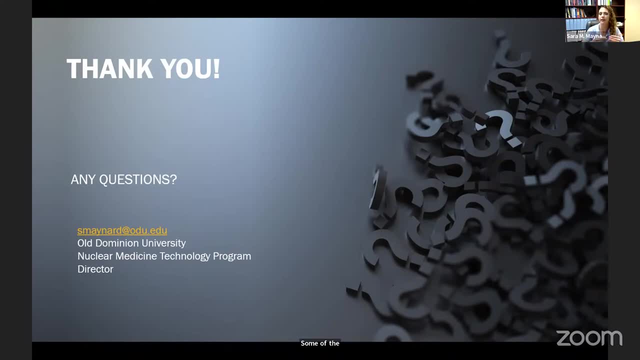 Um, cancers are not glucose avid like prostate cancer, and she tends to be more slow growing Um, so it doesn't take up as much of that radioactive sugar. So that's really where technology is going right now- is developing radiopharmaceuticals. 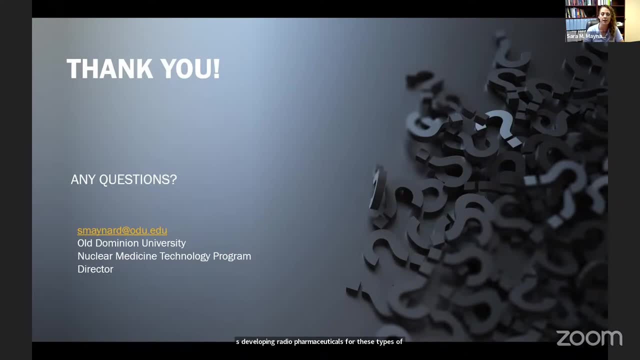 for these types of cancer that don't take up the glucose. So, um, a really, really cool one that actually two weeks ago I just got to be a part of on the Sentara Pet CT mobile. It's called Pilarify. 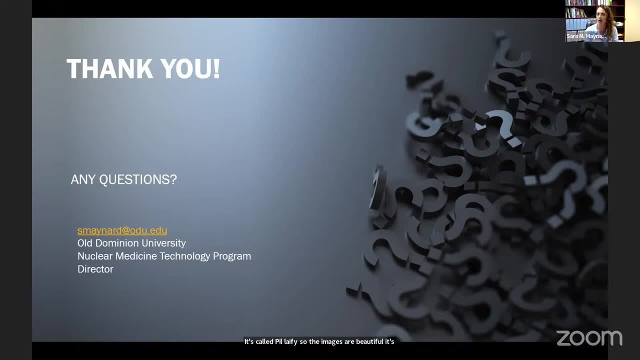 So the images are beautiful. It's designed just for prostate cancer, Um. so we've had like three breakthroughs in prostate cancer imaging agents in the last couple of years and it's honestly been a little difficult to keep up. We also have another one that's geared more towards um neuroendocrine carcinomas. 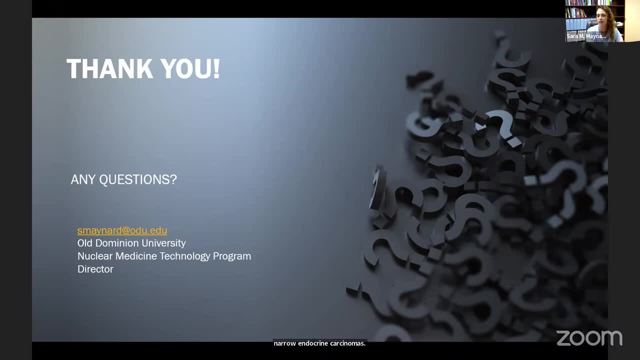 So what the researchers do is they look at the characteristics of these types of cancers and the types of cells that they have, And they try to create a radiopharmaceutical Um. so the radioactive materials, the part we're going to image, and the pharmaceuticals. 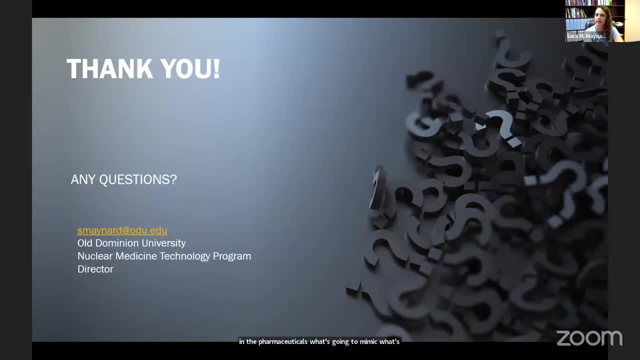 what's going to mimic what's going on with that cancer in the body So we can image it better, And that's it. The field is really taking off in that right now And it's it's really exciting that we're getting better images and better answers for. 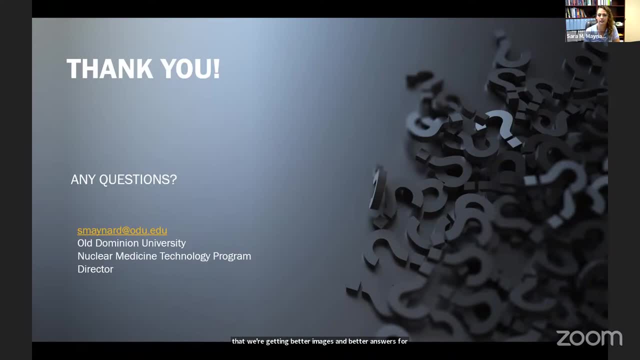 these cancer patients? Um? so I've got the um, I've got the first question. just to just as a reminder, if you want to, if you want to take it, you can submit your questions in the Q and a box on the bottom. 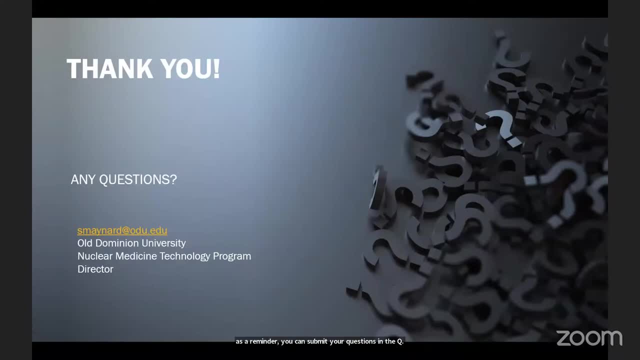 of your zoom screen? That was a really good question. Yeah, Sarah, maybe. um, especially since some of the students the what's this or you know what's this after the fact, do you have any references that might be useful for people? 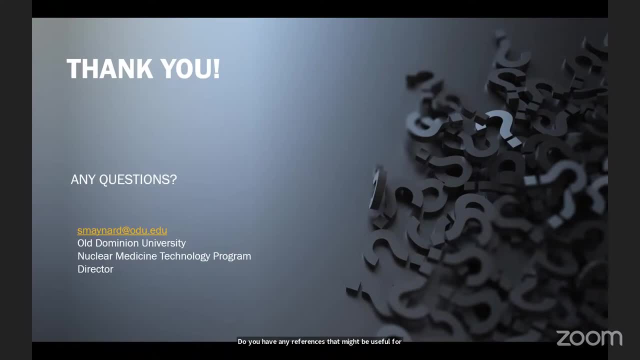 that want to, that want to listen to this, want to get started in learning more about this? Sure, So the Society of Nuclear Medicine and Molecular Imaging website has a ton of resources: webinars, videos. Also, YouTube is a really great resource that we've been referring our students to. I am a REIA's mentor. 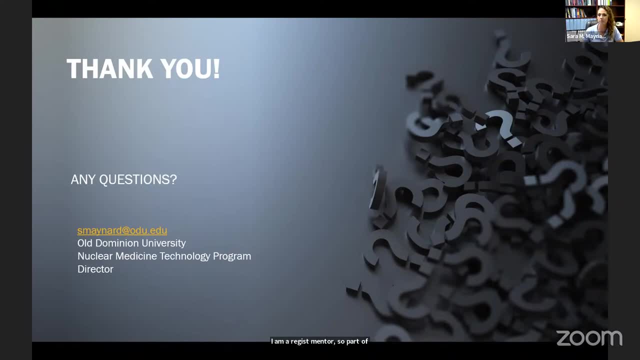 So part of my REIA's mentoring is showing inside a nuclear medicine department after hours when there's no patients. but we will be exploring some patient images as well. with the identifiers removed, So my contact information should be on the share screen If you'd like to. 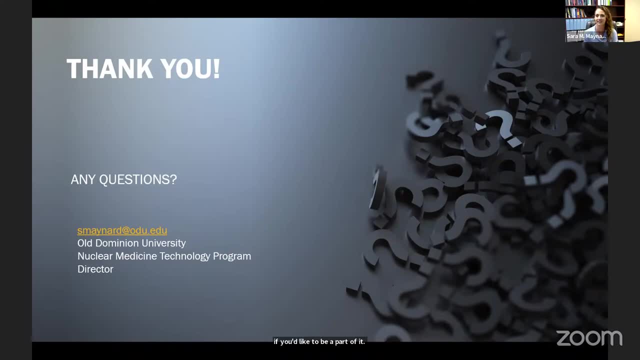 be a part of it. it's not too late, So contact me. That's awesome, Great Thanks, Okay, Maybe another somewhat related question. I mean, what drove you into this field? What was the thing that made you interested in it? So my mom's a nurse and my dad is an engineer. 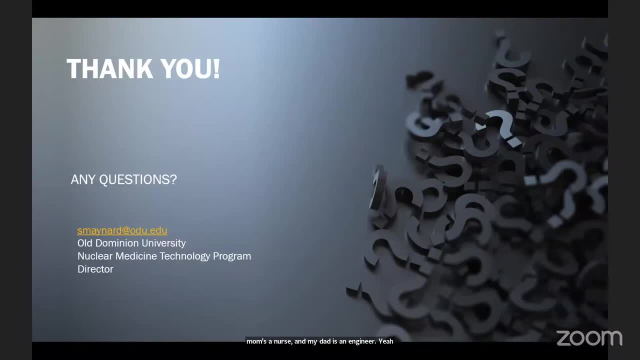 and I tried a little bit of both in undergrad. Nursing wasn't a hundred percent the right fit for me, and neither was engineering. I really liked engineering, but I missed the caring for myself. So I really liked engineering, but I missed the caring for myself, So I really liked. 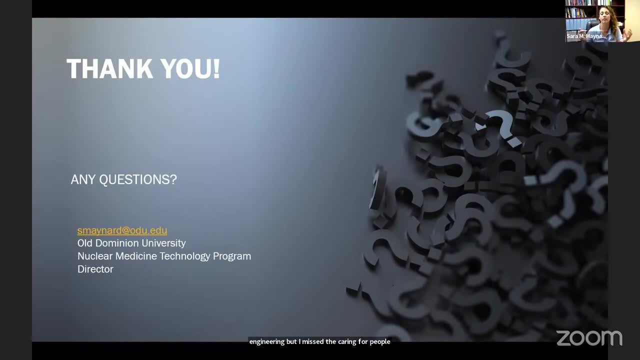 people aspect of it. So nuclear medicine really combined my two interests. for me I'm still taking care of patients but I enjoy the longer studies. I enjoy thinking critically about what I'm doing with the studies and what the images are doing and what my calculations are. 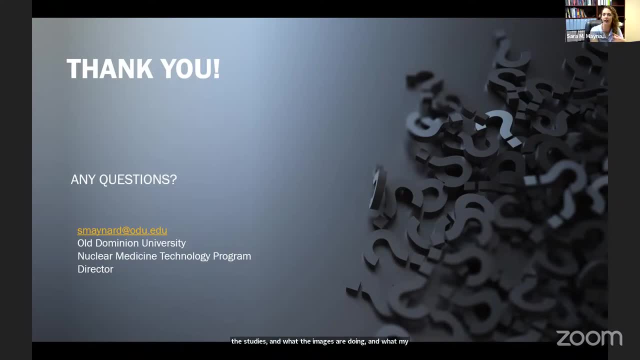 saying- And it's very- I find it very- rewarding working with cancer patients or heart transplant patients that I see on a repeated basis, over and over. Yeah, that's great. Yeah, One of our students. when I announced this talk, he mentioned that you know he was looking forward to seeing it. 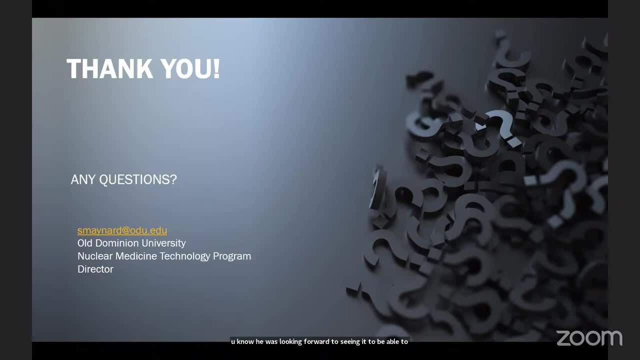 to be able to tell his family why nuclear physics is actually useful. I could see why you would be interested in it, So that's great. Thanks. Yeah, There's so many places that you can go with it, So nuclear medicine just depends on where. 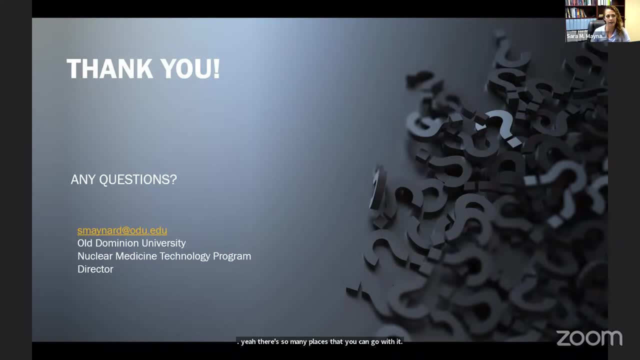 you go to school. Some places it's an associate's degree or a certificate. In Virginia it just happens to be a bachelor's degree, But a lot of people use that as a starting point to go on to be health physicists and actually do the calculations for these cancer treatments, or 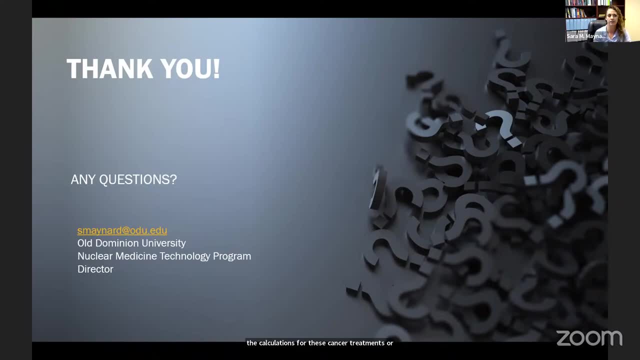 calibrate the equipment to become physicians, to become physician's assistants, to become licensed pharmacists who elute the generators of radioactive materials and compound the radiopharmaceuticals, to give to us Lots of different exciting directions that you can take, just starting out in nuclear medicine. Yeah, that's fantastic. Thanks, Yeah, And one more. 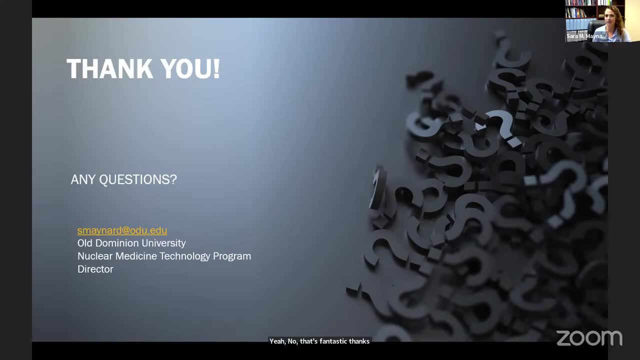 thing, One of our program graduates is actually the manager of the new Theranostics department at Johns Hopkins, So they are studying the relationship between these diagnostic radiopharmaceuticals and therapeutic radiopharmaceuticals and working to develop new ones. 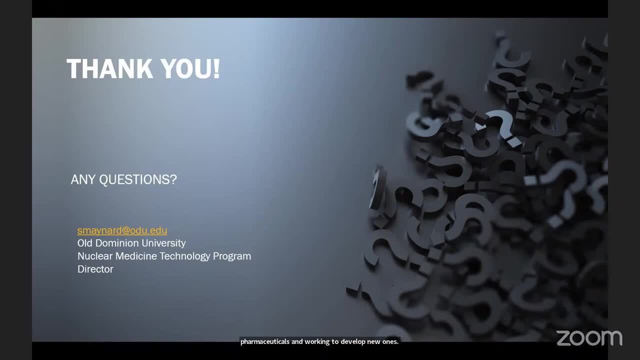 That's exciting, Yeah, very exciting. Well, I mean, if people don't have questions in the live session, they're your emails right there So they can bombard you with all the follow-up questions, right? Absolutely Well. on behalf of Old Dominion University and the RAISE program planning committee. 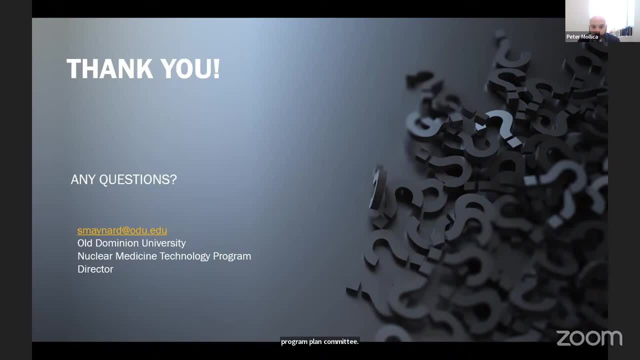 I would like to thank you, Sarah, one more time for joining us and sharing your professional journey. We're going to follow it. It's really interesting. I mean, even for non-clinicians, it's a very interesting and exciting field, And 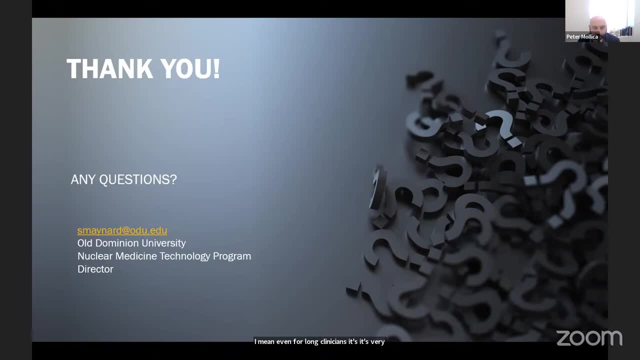 yeah, It's awesome kind of seeing how STEM plays into health care, Because, you know, health care is an issue. But I would also like to extend my gratitude to ODU's Office of University Communications and the Office of Distance Learning for their support and their help. 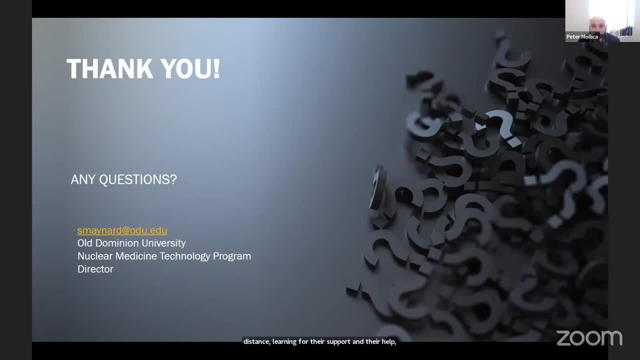 in getting these events up and running and then getting it out to the students interested. Thank you, And to our audience. thank you for tuning in. For more information about our free virtual summer program, you can visit oduedu slash Reyes. Today's session has been recorded. 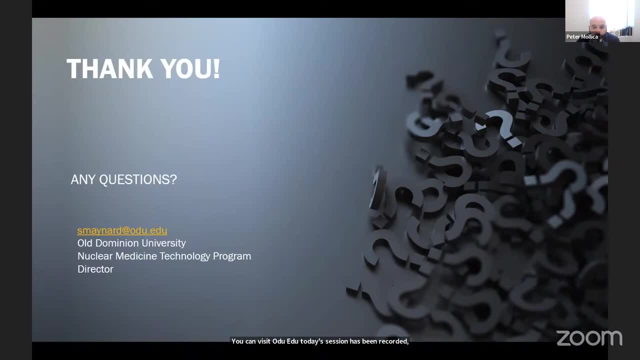 And if you'd like to watch it again or share it with your friends, you can access it from the Reyes website at oduedu slash Reyes. And if there are no more questions, this concludes today's program, So please have a wonderful rest of your day. And thank you again, Ms Sarah Maynard.